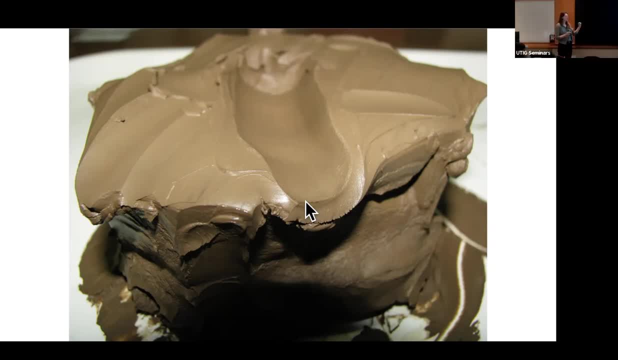 It's pelagic clay. It's visually homogenous. It's like ooey brown, very fine grain. Mineralogically it's smectite, zeolite and some iron oxides, So very hard to tell. like what's in it visually. 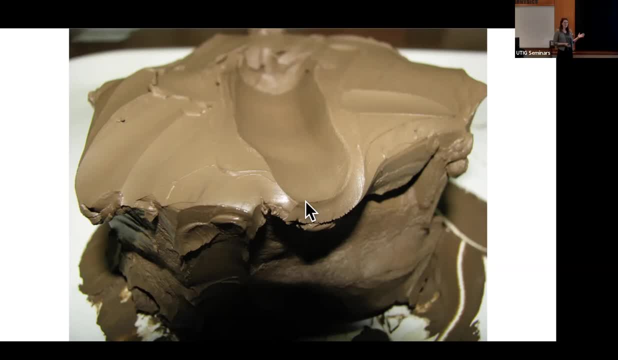 And a lot of paleochenography. Paleochenographers avoid this type of sediment like the plague because there's no microfossils so it's very hard to date. It accumulates really slow sedimentation records or sedimentation has really slow sedimentation rates so you can't get high-resolution records. 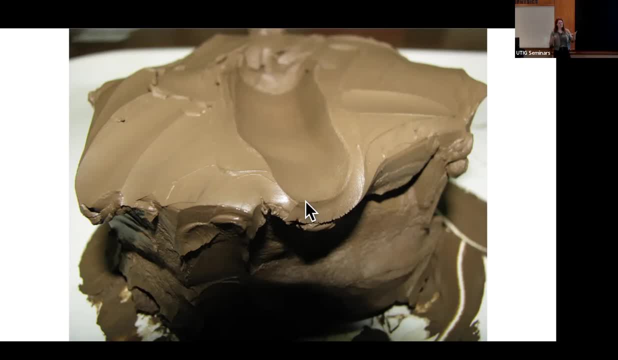 And it sits at the bottom of the seafloor for a long time and interacts with seawater, so everything gets altered. I think that those are three of the biggest assets of these clays. The slow sedimentation rates allow for really long records of sedimentation. 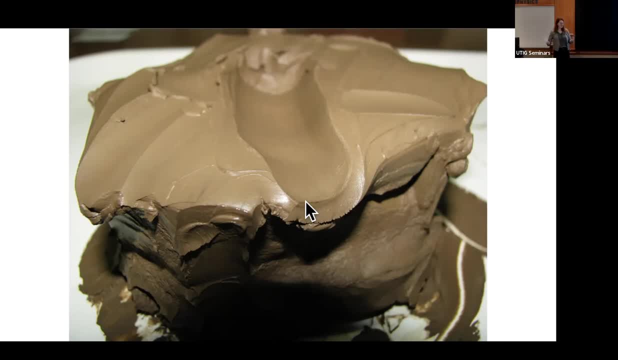 So we're going to be looking at the entire Cenozoic today, 65 million years ago or even far back as 95 million years ago, And the altered nature of the sediment also allows us to look at how sediment interacts with ocean chemistry and what that means for climate and ocean chemistry. 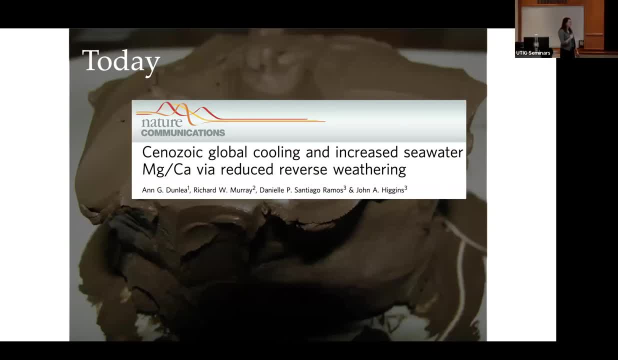 So the project I'll be talking about today is published in Nature Communications. in this publication, I've done a lot of work since then, but for this talk and this audience, I thought this would be the most interesting, so I'm excited to be presenting this today. 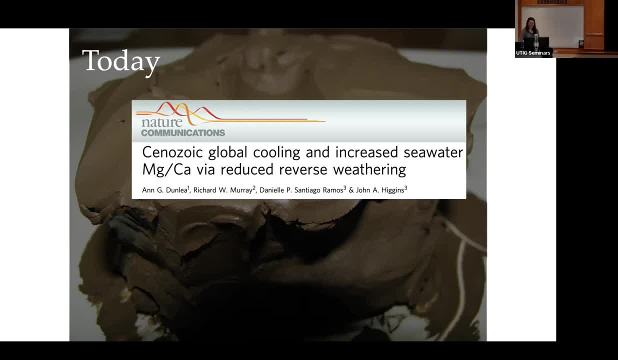 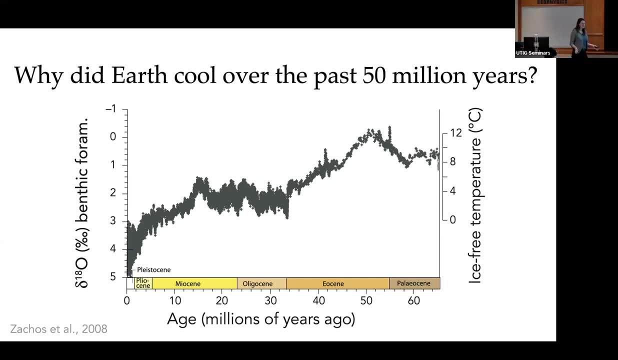 And I'll touch upon a few ongoing projects that have stemmed from this work at the end. So, to start us off, we're going to look at one of the big geologic mystery in Earth's past: why did the Earth cool over the past 50 million years? 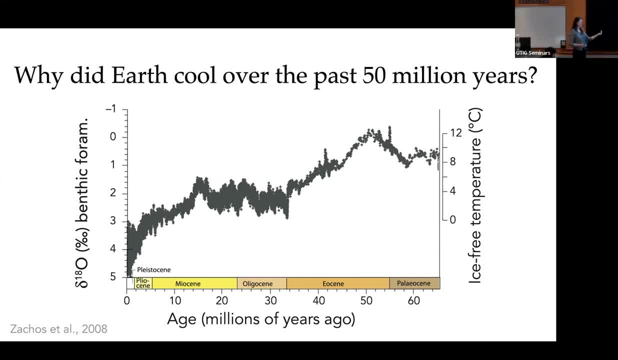 So on the x-axis here we have age of millions of years ago, on the left is the present and on the y-axis is a delta 18 oxygen isotopes record from benthic foraminifera looked at over time. So this delta 18 O is affected by sea ice volume and temperature. but if you remove the effect of sea ice broadly, 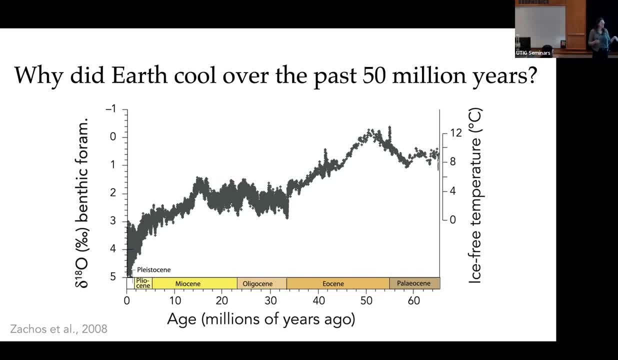 the right axis shows the ice free temperature recorded by this proxy. So there's been a decrease in temperature from 50 million years ago, when we were a greenhouse, to more today, where we have ice sheets in the polar regions And what we call an ice house. 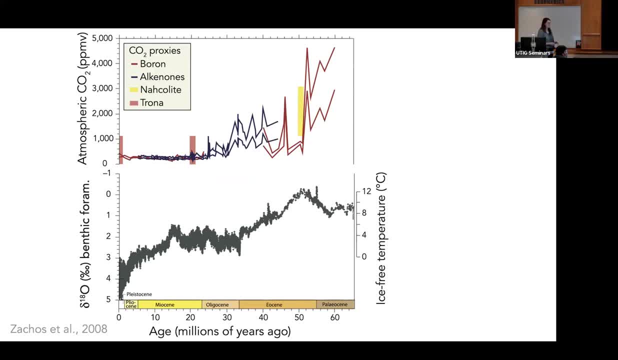 So this cooling has broadly been linked to a decrease in atmospheric CO2, so the top plot has the same x-axis and estimates of atmospheric CO2 concentrations from a variety of proxies that widely disagree with one another, but overall they're shown a decrease in carbon dioxide. 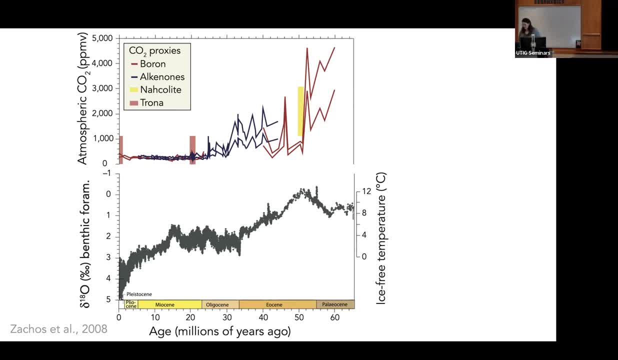 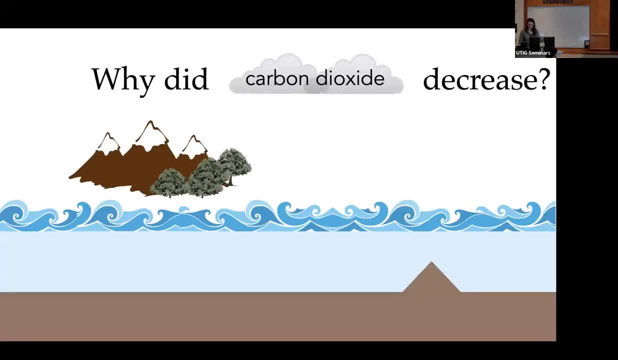 over the Cenozoic. So then, the question is: why did carbon dioxide decrease over the past 50 million years? So there's many hypotheses as to why carbon dioxide decreased. One hypothesis says that there's decreased seafloor spreading, so there's less volcanic outgassing from the Earth's mantle, and that has caused a decrease in atmospheric CO2.. 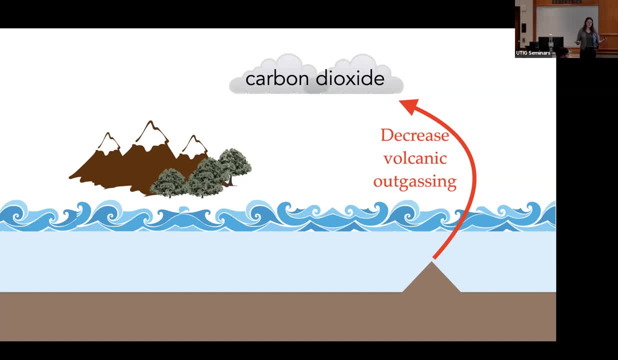 However, if you look at the estimates of the rate of ocean spreading rates, there's a whole bunch of estimates. Some say it's increasing, some say it's decreasing, some say it's remained constant. So the jury is still out on exactly what ocean spreading rates and volcanic outgassing 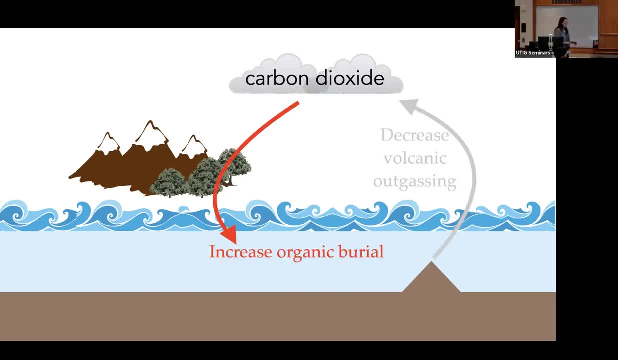 have did over this time period. Another hypothesis is that there is increased photosynthesis, and the photosynthesis drew CO2 out of the atmosphere and increased the amount of organic matter buried in the ocean. But exactly where and how this massive amount of organic matter is buried in the seafloor is still 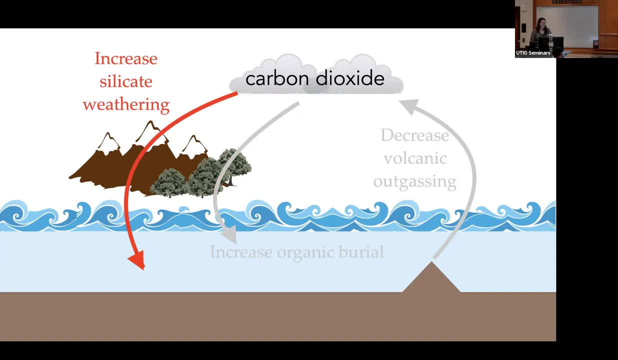 not totally figured out. There's still questions surrounding that. And a third hypothesis is that there is an increase in silicate weathering over the Cenozoic. that pulled CO2 out of the atmosphere, And so there's popular hypothesis like the uplift weathering hypothesis, or you can increase the weather ability of continents. 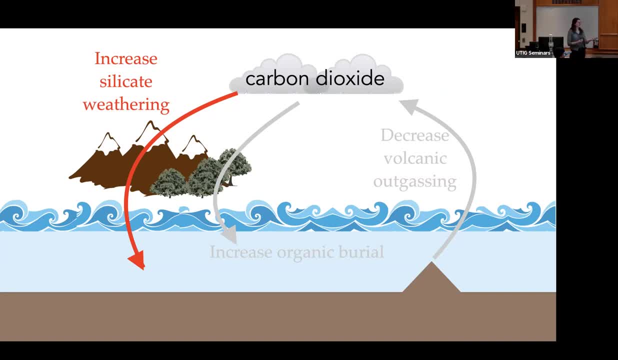 And increase silicate weathering, which will draw down CO2.. So there are some issues with this hypothesis also that I will get into shortly. But broadly, all of these hypotheses kind of have thorns in the side of them, So there's room still for other processes that may be affecting this global CO2 decrease. 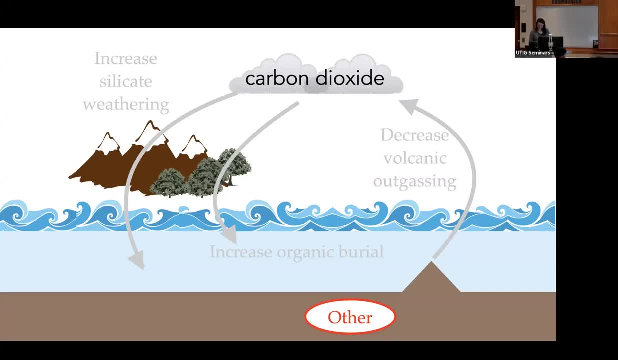 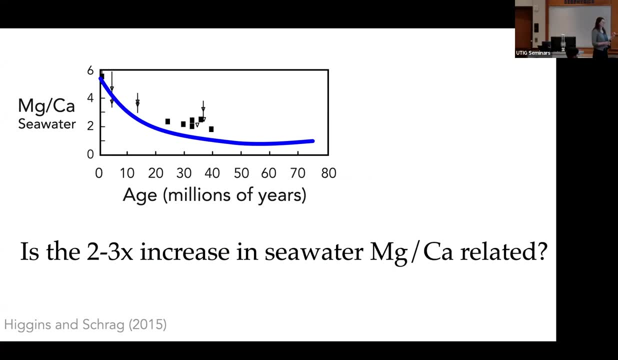 And that's what I'll be talking about today- is another hypothesis. Before I get into the silicate weathering hypothesis and this other hypothesis, I wanted to point out one other trend in that happened over the Cenozoic. In this plot we have age of millions of years on the x axis and the magnesium calcium ratio of seawater on the y axis, and 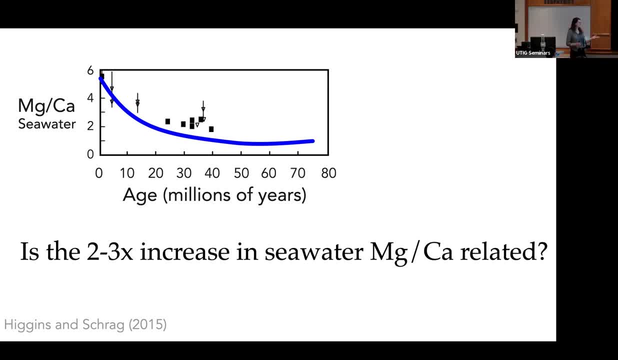 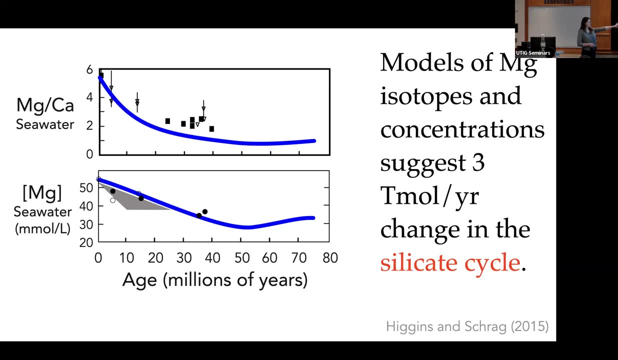 broadly. a variety of archives have suggested that the magnesium calcium of seawater has increased Two to three fold And that is likely due to an increase in the magnesium concentration of seawater. So this is another map or another plot, with the same x axis and then on the y axis is magnesium concentrations of seawater. 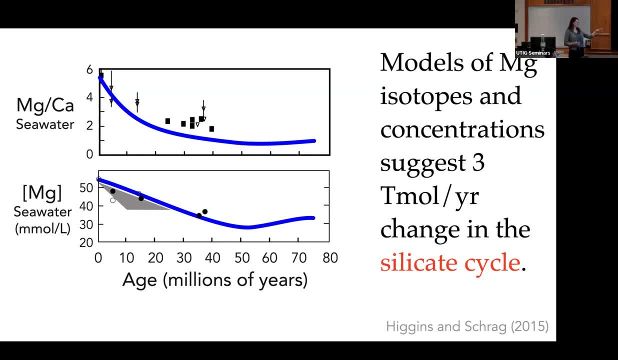 And models of magnesium isotopes in Higgins and Tragg 2015, and the concentrations of magnesium suggest a three teramole per year change. that's related to the silica cycle. so the other option would be that you change the carbonate cycle. that changes the magnesium and calcium. 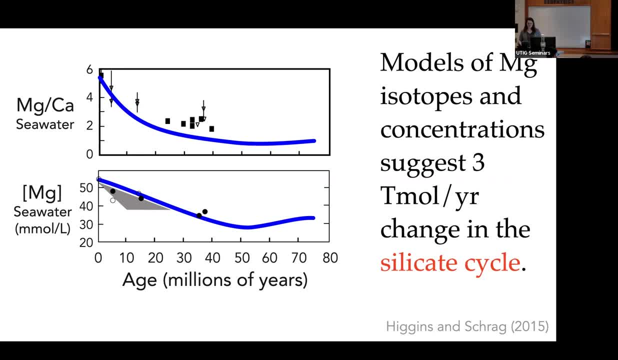 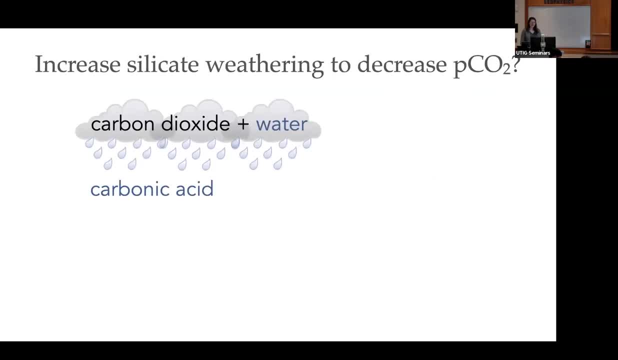 properties, but the magnesium isotopes suggest that it's a change in the silicate cycle. So since this is related to the silicate cycle and the silicate weathering hypothesis is related to the silicate silicate, let's dive into that a little bit deeper. so the increase in silicate weathering hypothesis that is thought to have decreased CO2 goes like this: 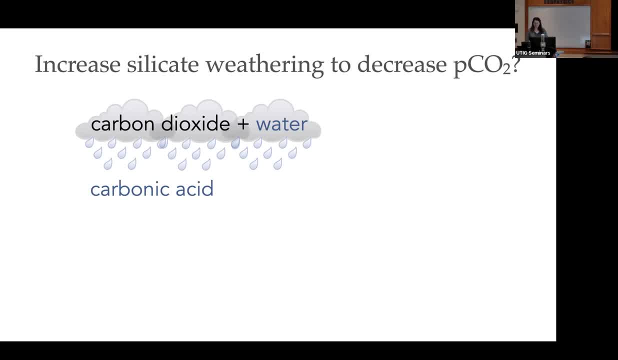 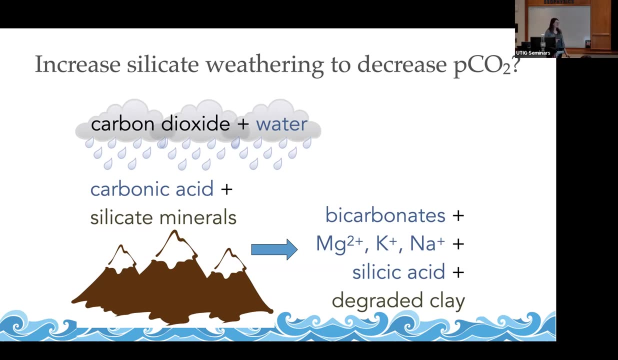 You have carbon dioxide in the atmosphere. it combines with water to form carbonic acid. That carbonic acid rains out or interacts with silicate minerals, such as like in any typical rock, And weathers away bicarbonates, magnesium, potassium, sodium, ions and silicic acid, and all of those get washed out through rivers to the sea, leaving behind a degraded clay mineral. 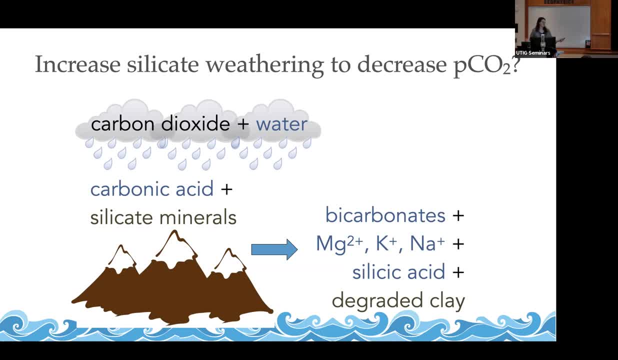 So this is a weathering reaction that you may have learned about in various classes, And that is how you get CO2 from the atmosphere into the ocean and so that the hypothesis that you can uplift mountains to increase the amount of weathering that happens. 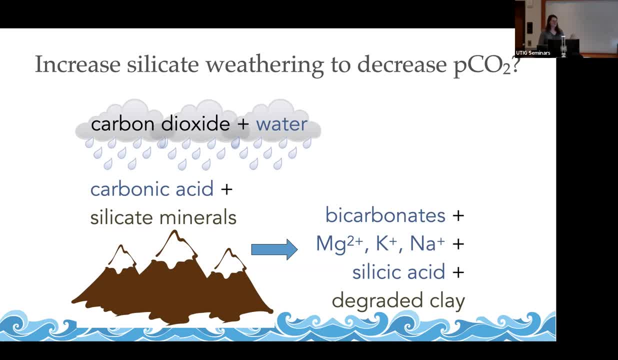 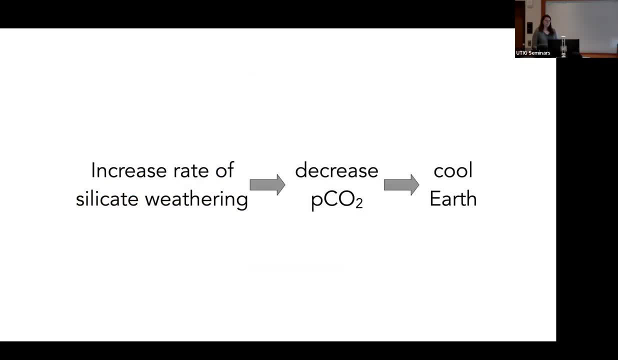 Or you can change the weather ability or where your continents are positioned. there's lots of ways you could possibly get an increase in silicate weathering to decrease CO2. But one one kind of thorn in the side of this hypothesis that complicates this idea is that if you increase the rate of silicate weathering and decrease CO2 and cool the earth, 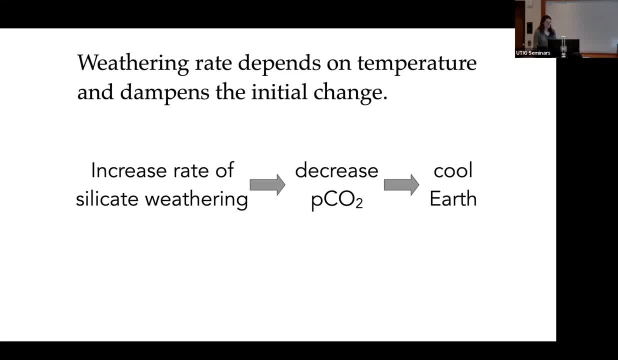 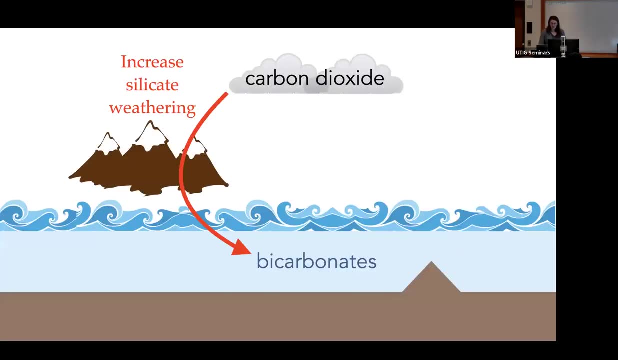 The initial chemical weathering of silicates is temperature dependent and so if you cool the earth you can actually decrease silicate weathering And kind of dampen the effect of this process and like slow it down. The other issue with this hypothesis is that 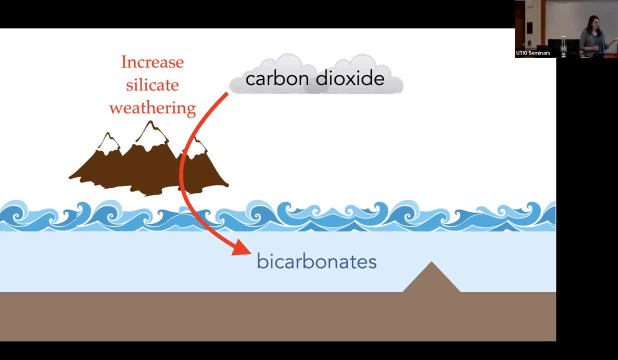 If you increase silicate weathering, you're going to increase the amount of bicarbonates that are deposited in the ocean and if you Continue, if you just increase, you turn the lever for silicate weathering and just increase it with nothing else changing- you're going to completely deplete. The atmosphere of carbon dioxide within a couple million years. so you can't just turn up in like silicate weathering and have nothing else change. you have to have something that's returning CO2 back to the atmosphere and establish a new steady state. 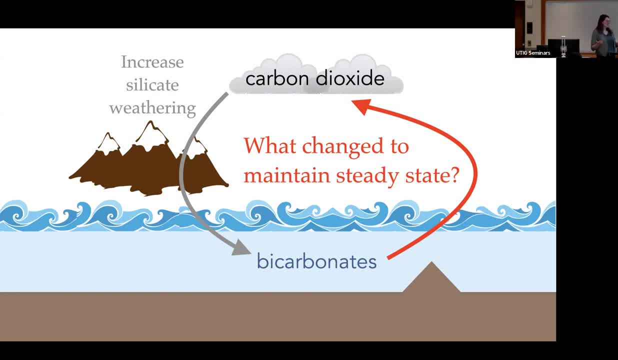 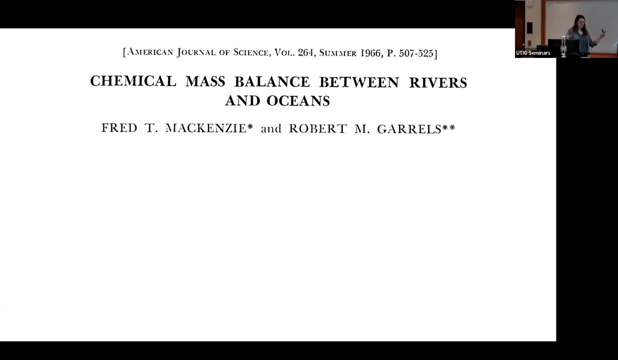 So the question is like: what changed Aside from increase in silicate weathering to maintain the steady state? And so, To look at that question, we're going to take it back, we're going to zoom out a bit and look at big ocean budgets and like where, where do the carbon? like where do bicarbonates go? like what, what is what? where do all these elements from weathering go? 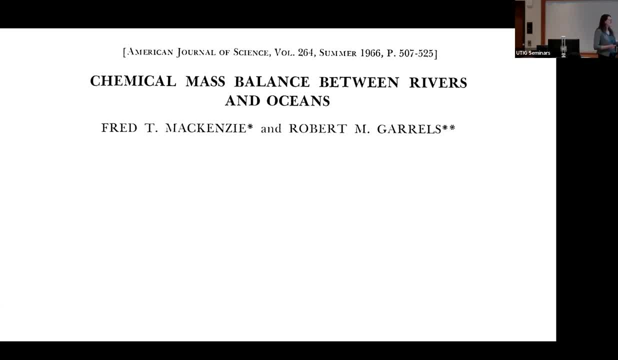 So in the 1960s mccarroll and genzy, mckenzie and garros did a giant mass balance calculation of the river inputs and Ocean outputs, Trying to figure out balance like where everything that's coming in is going out. 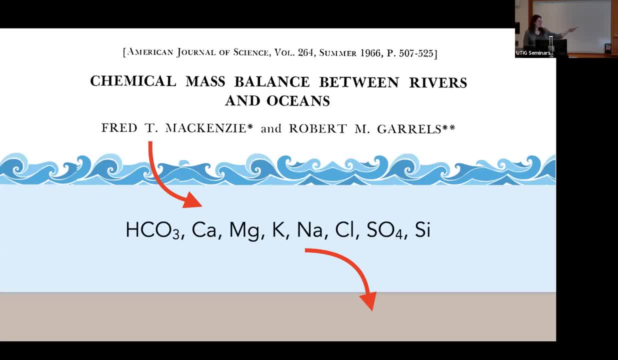 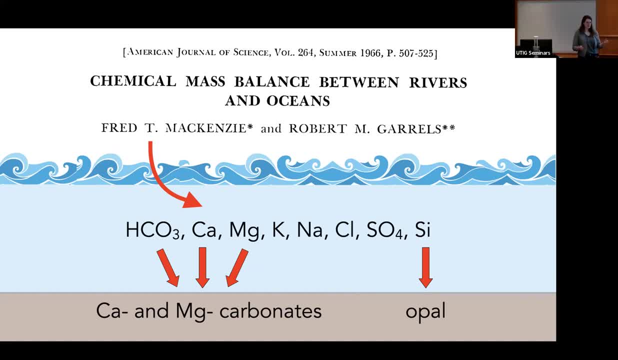 And most of the silica could go into opal like biogenic silica, so that took care of that. but there's still a lot of magnesium left that was unaccounted for, with no supposed sink, along with potassium and sodium. So the question was like: well, 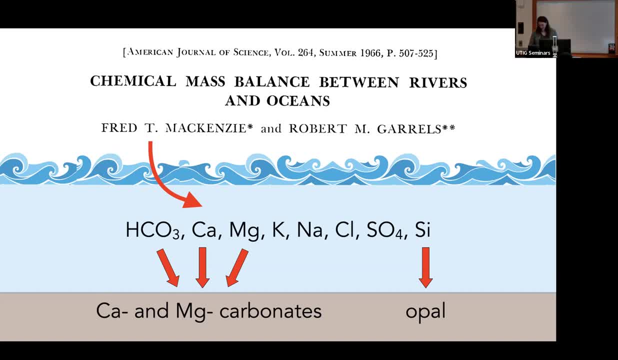 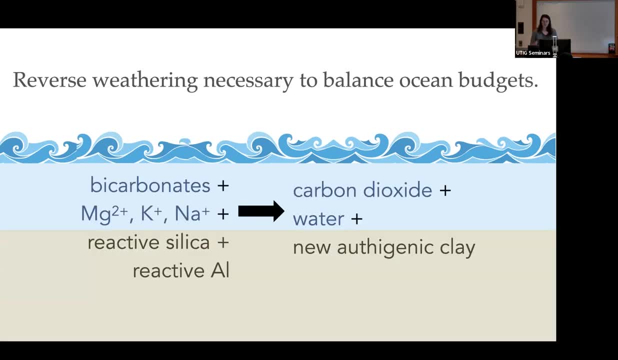 Where did those elements go? And so, in order to balance this budget and figure out where these elements are going, they hypothesize a reaction that they called reverse weathering. So reverse weathering is the exact opposite of the weathering reaction we went over a couple slides ago. we have bicarbonates in the ocean, magnesium, potassium, sodium ions in the ocean. that combines with reactive silica, so perhaps in biogenic silica and a reactive aluminum. 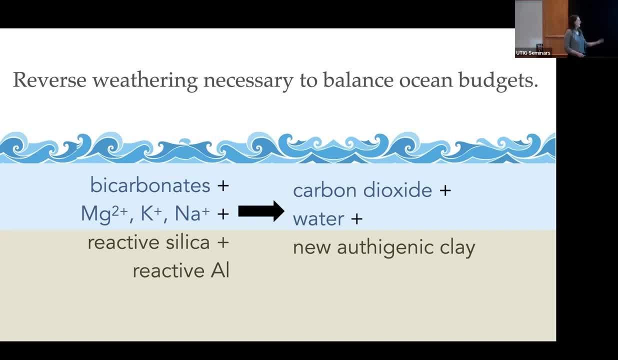 Maybe from rivers Or dust or volcanic ash, and all of these can combine to form a new authentic claim there. also, cation is being taken up into a claim in our, and the bicarbonate is being converted back to CO2.. And so this kind of reverses what the weathering reaction does, and it is able to account for the uptake of these cations into the seafloor. 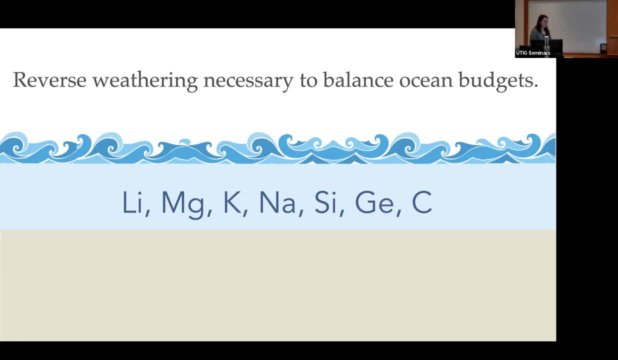 And there's been a lot of work that has been done since McKenzie and girls and hydro thermal events were discovered which introduced a huge sink of many elements. But to this day, reverse weathering or some kind of low temperature authentic process remains a very necessary part of all these elements- ocean budgets, so this is still like an important process. 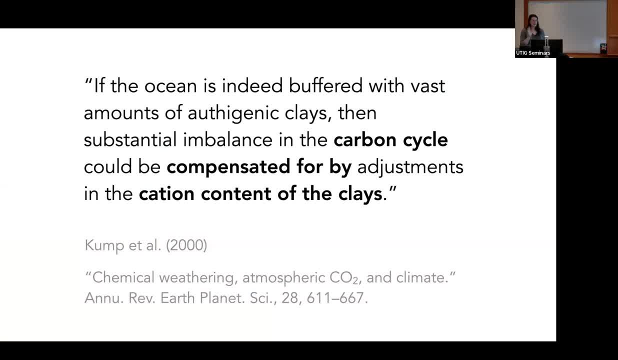 it's Yes. and in terms of balancing an increase in silicate weathering, I This is a quote from a paper by come pedal in 2000, where they were looking at what might balance An increase in silicate weathering or other ocean processes. and they said: if, if the ocean is indeed buffered with vast amounts of authentic clays. 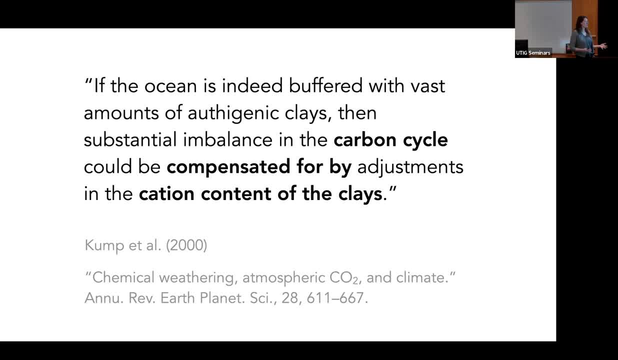 Then substantial imbalance in the carbon cycle could be compensated for by adjustments in the cation content of clays. so I like this quote because it seems like he's a little skeptical, like if indeed it's buffered, but But also really points to the importance of this authentic clay sink and in terms of balancing the carbon cycle on a global scale. 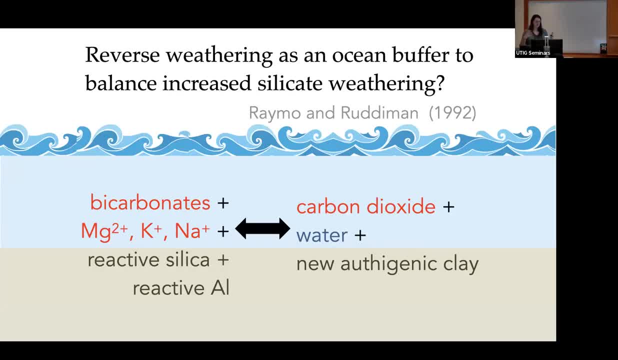 And so this is one of the ways: reverse weathering, or this cat and uptake into clays is one of the mechanism that a well known paper by Raymond rudiman suggested balancing their budget. so, Raymond rudiman are- I guess it's a famous paper- for uplift weathering, you uplift the. 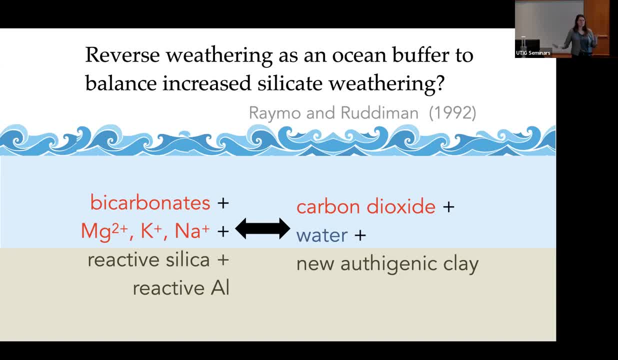 Himalayans increase Silicate weathering and they knew that they needed something to balance the input of bicarbonates to like maintain a new, steady state. so in their paper they say that: Oh, if you increase the amount of bicarbonates and ions from. 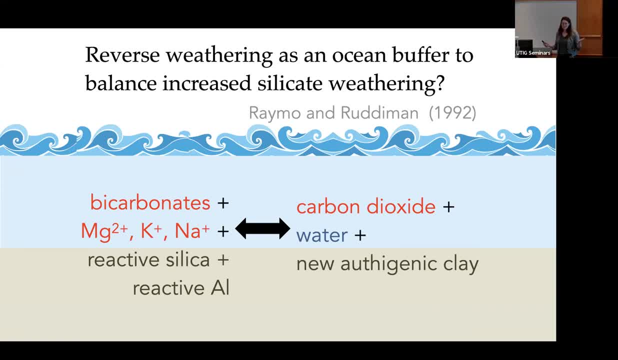 Silicate weathering, then you'll form more authentic clays and CO2 will be returned to the atmosphere and you will balance your budget. However, everyone- These papers all- kind of wave their arms and be like, yeah, there's probably plays down there, they're probably doing something. 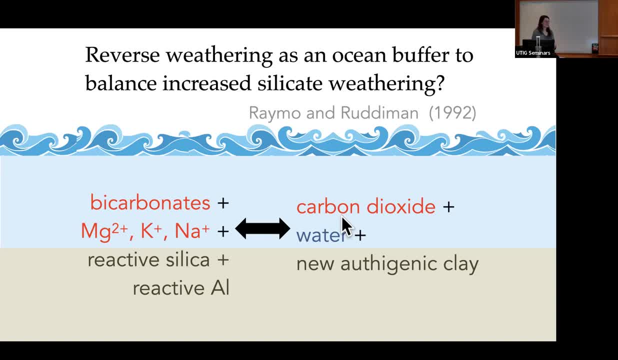 But these clays have kind of remained really elusive because they're so hard to identify. they look an awful lot like other clay minerals in the ocean that aren't authentic. They can get diluted by a lot of biogenic material, so actually finding evidence for the sink is exceedingly difficult. 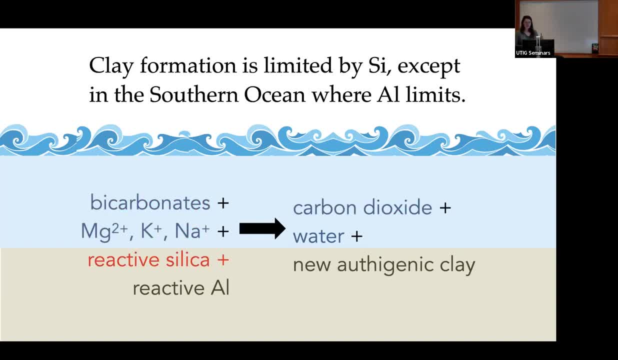 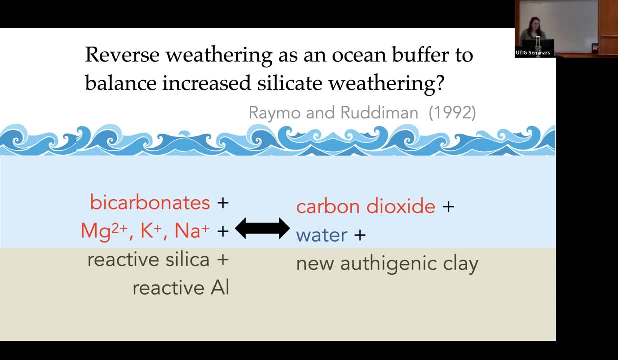 But there has been. Oh yeah. and the other thing I want to point out is they. they said if you increase bicarbonates you'll get more clays. The few studies that have identified clays in near the Amazon delta or in the southern ocean have shown that reactive silica is actually what's limiting the formation of these clays. 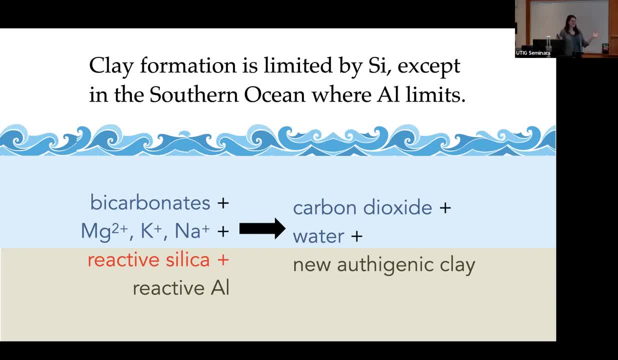 In most of the world's ocean, so there's bicarbonates everywhere. that's easy to find, but silica is Under saturated in the ocean, and so if you added more silica to many parts of the seafloor, you have all these other components that you need, and so you can form a new clay mineral. 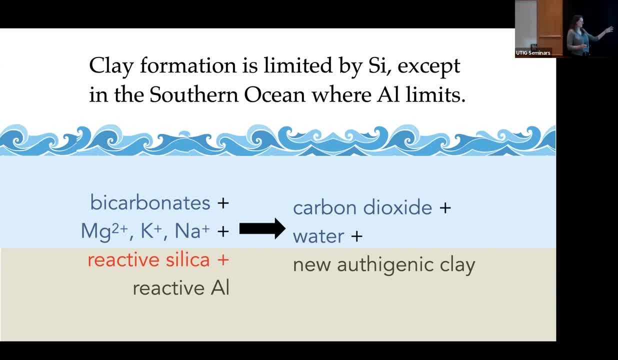 So reactive silica is actually like the limiting reactant in this process. the only place that's not true is in the southern ocean or other silica rich sediment deposits. So their hypothesis that this will just balance it might not work exactly, because silica can limit this reaction. 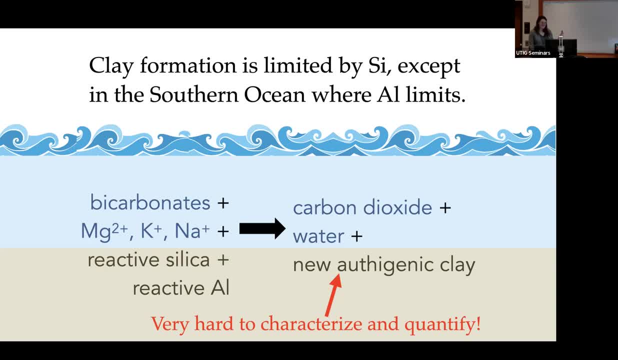 And I mentioned before that the these clays are very, very hard to identify. There has been SEM images and some poor water, a lot of poor water evidence for them, but actually figuring out how much of these cations are taken up into these clays is is quite challenging. 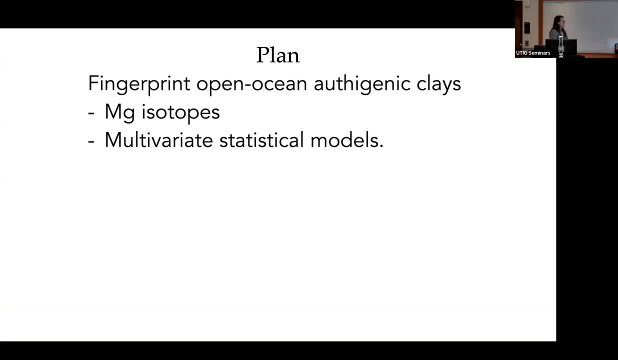 So that's what we'll do today, Today in this talk. for the rest of the talk, i'm going to go over two methods we use to identify the These clays- magnesium isotopes and multivariate statistical models- and then we'll extrapolate our results to a global scale and see how important this othogenic clay sink is that we're we identified. 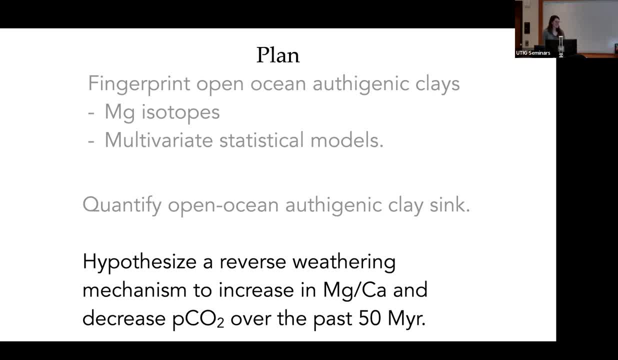 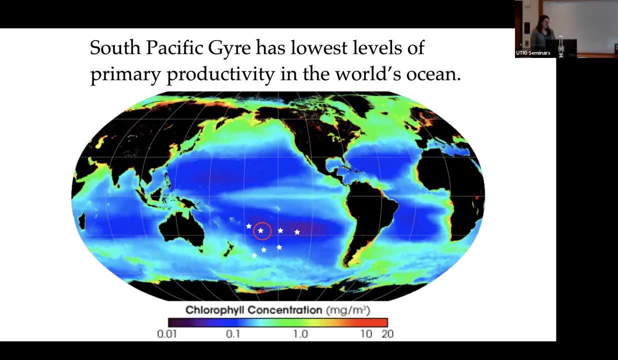 And then we will move into talking about a hypothesis that reverse weathering changed and that may have decreased the atmospheric CO2 and increased magnesium calcium over the Cenozoic. and that's our roadmap. So, to start off, we're going to go where. 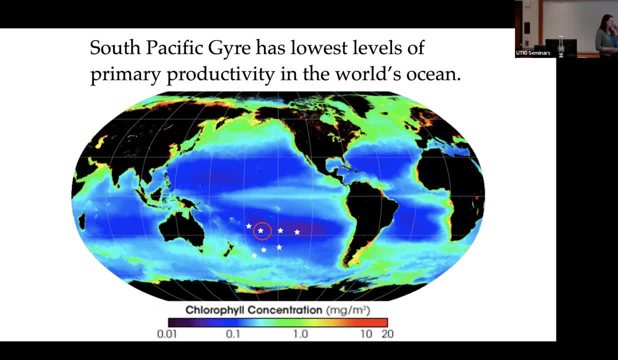 There is a very high concentration of othogenic minerals and we're going to go about as far away from land as you can get, in the South Pacific gyre. so this background math is chlorophyll concentrations, which is a proxy for primary productivity, and the South Pacific gyre. 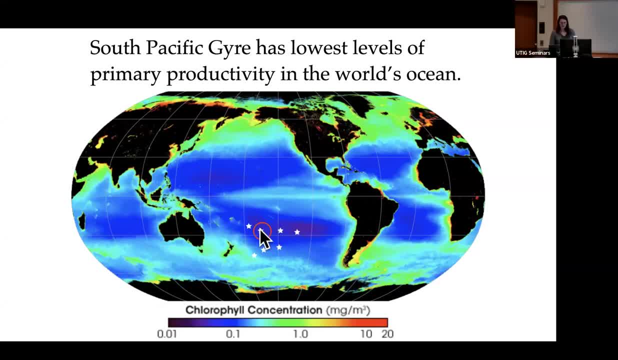 These are the seven sites that I had analyzed or analyzed, and today we'll be talking about this site in The circle. The circle in red and this purple area in the map is some of the lowest chlorophyll concentrations in the world, and so this is where. 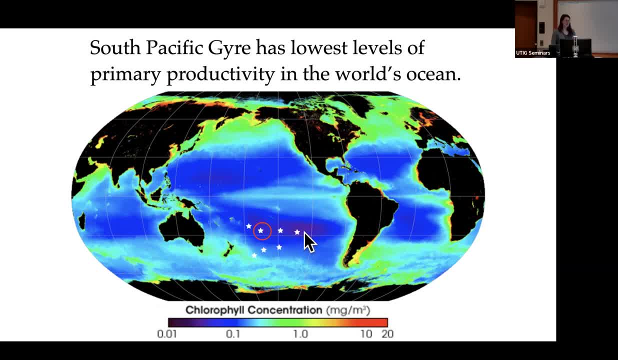 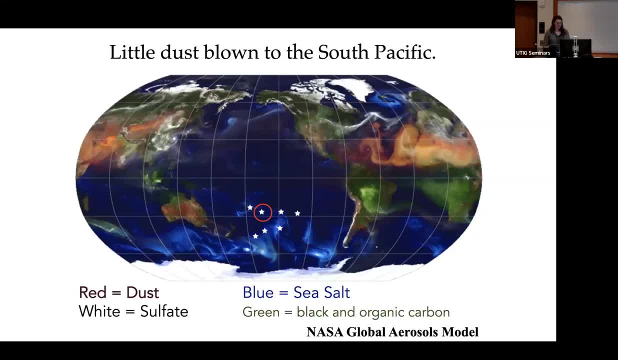 Primary productivity is extremely low, which means there's very little biogenic material to dilute our othogenic clays. there's also very little dust. this is a NASA aerosol simulation of Global aerosol simulation by NASA. that Where all that we really want to look at right now is the red or the orange ish color which represents dust. so the northern hemisphere has orders of magnitude higher dust fluxes than the southern hemisphere. 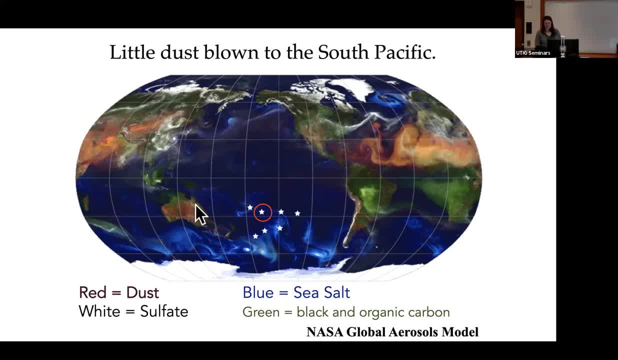 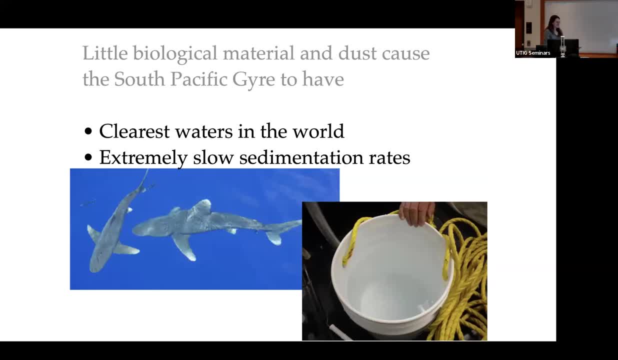 Where Australia is the biggest source of dust, but it still is not very much so out in the middle of the gyre, very little dust, So little biological material and little bit of dust. the South Pacific gyre has some of the clearest waters in the world and extremely slow sedimentation. 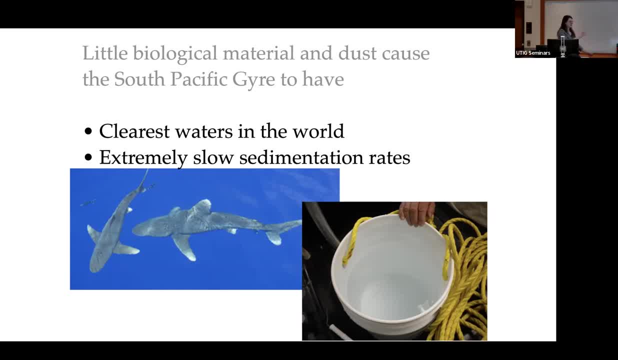 rates. I think these sharks were like 14 or 15 feet long and they could see them like all the way down in the ocean when they were like this big, like at depth, And then they were like, oh, it's a little fish, and then it swam up and it was like a massive shark. 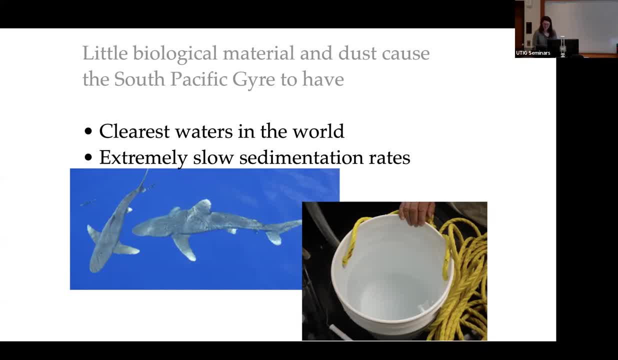 So just the visibility, unbeatable. Oh yeah, and I guess another thing: sedimentation rates here are about One meter per million years, so on our time scales that's about one micron per year, And I want you to think about that next time you sleep under your bed, because dust definitely accumulate there faster than it does in the South Pacific gyre. 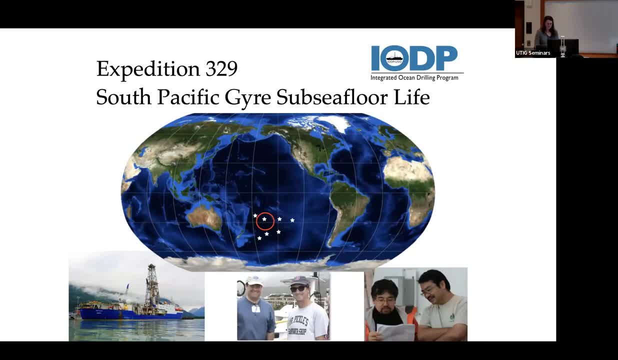 So very, very, very slow accumulation rates. So the sites in this study were collected during the integrated ocean drilling program, now the international ocean discovery program Project In the South Pacific gyre expedition 329 it was. the cruise was targeting microbiology. so what kind of life lives in these extreme remote environments? 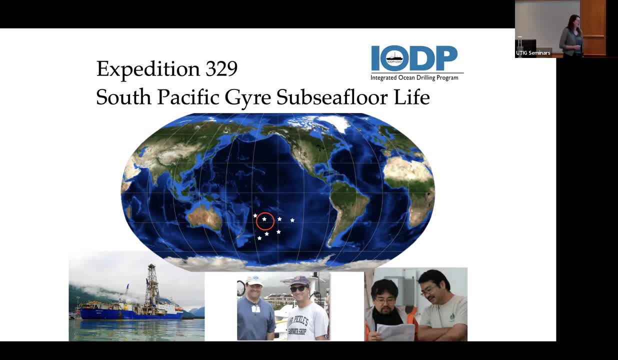 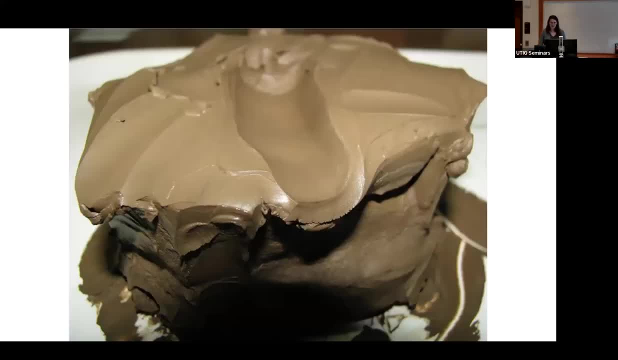 Was coaching by Steve don't and whom you in a gaki son and I appreciate advisor rick Murray was on there And the type of sediment that they recovered predominantly looks like this: very, very hard To date to see any different mineralogy, mineralogical changes, because it's all been altered. 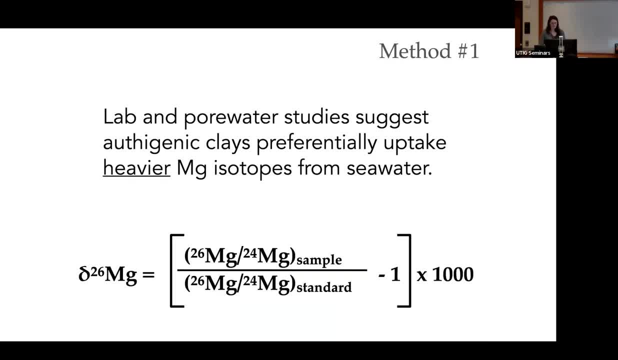 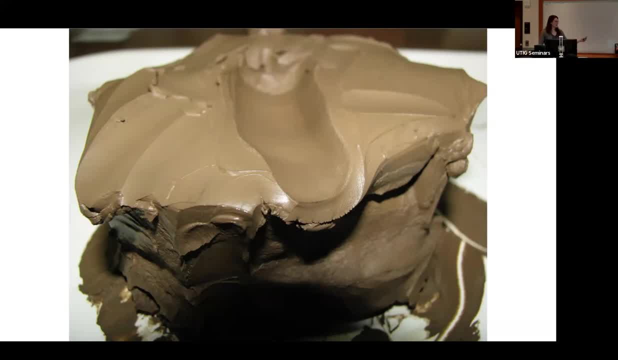 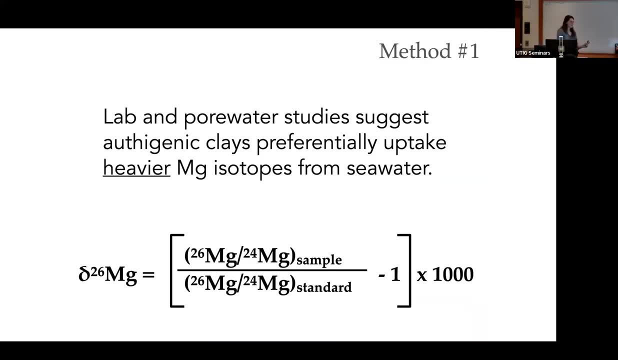 But chemically we found it to be quite diverse, And so we just we took the sediment, dissolved all of it in Various techniques- flux fusion, acid digestions- and analyze it for magnesium isotopes. and then i'll get into the second But the first method. 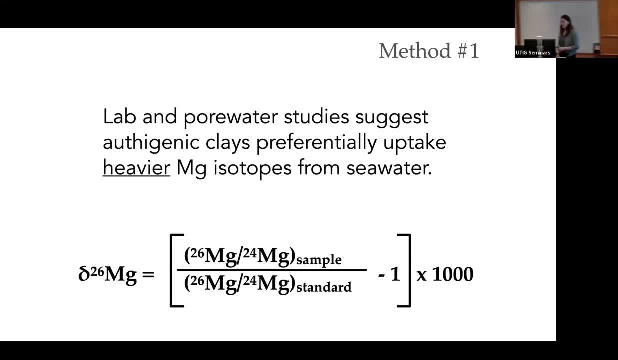 The second method is to take a little bit of magnesium isotopes. here at the bottom I have the delta notation for magnesium isotopes. But all that you need to remember for this talk is that there are lab and pour water studies. That suggests the oxygen acclaves. so when magnesium gets taken up into an oxygen acclaves it preferentially takes up the heavier magnesium isotopes. so heavy magnesium isotopes. 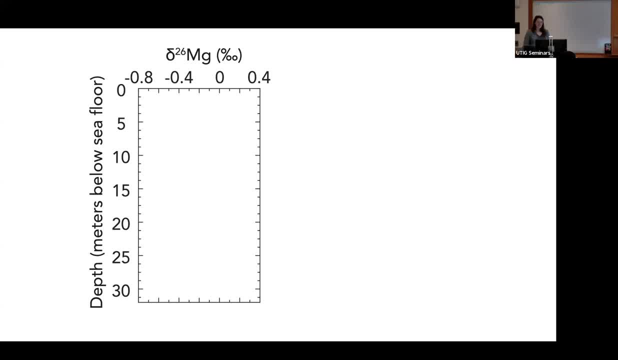 Probably not the genic. That's all You need to take away from this. So if we look at our data from site 1366 and the South Pacific gyre on the y axis, we have depth in meters below sea floor. For reference, this is drilled down to basalt and it is 95 million year old basalt, so that 30 meters of sediment accumulate in 90 million years. 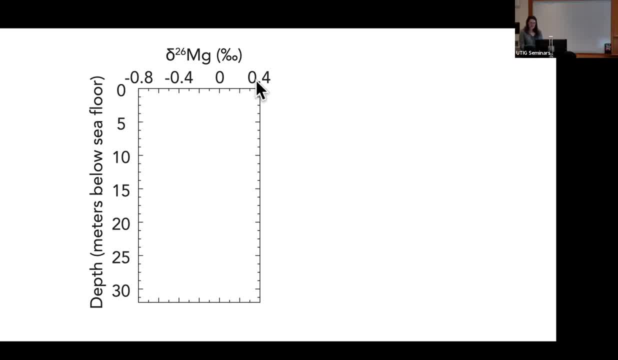 Very, very, very slow. And then on the x axis is the magnesium isotopes that will look out for the site. Our samples had magnesium isotopes signatures of seawater. they should plot near this purple bands And if they have the magnesium isotopes signature of continental material or dust they should plot near this band or in this band, and the data from 1366 show that near the top. 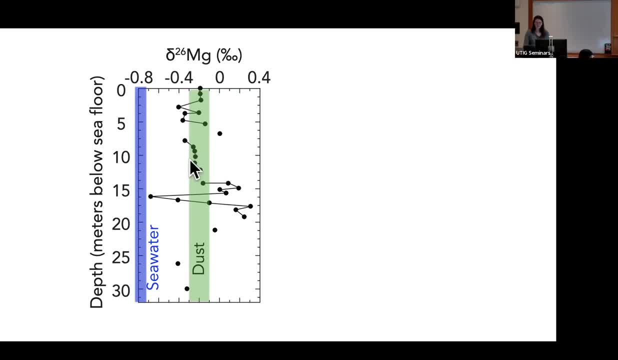 It does plot within the screen band. there's probably a lot of dust here. We have a couple of outliers that maybe there is a lot of seawater that was still in that sample when we tried it down, Analyzed it. but all of these samples have magnesium isotopes that are heavier than continental material. 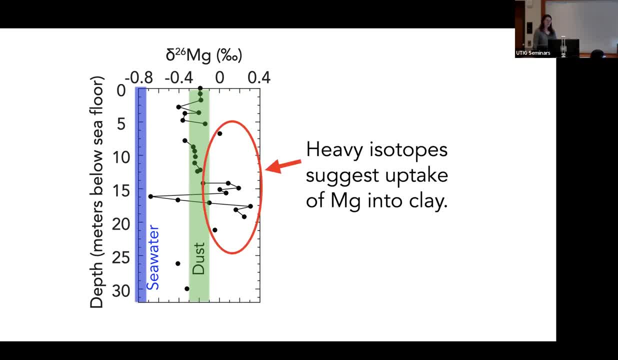 And we can interpret that. there's not much else that would explain this aside from An uptake of magnesium into an authentic clay mineral. So this is a beautiful few samples that are like have almost exclusively authentic material that Is undiluted by biological material, all the other stuff and 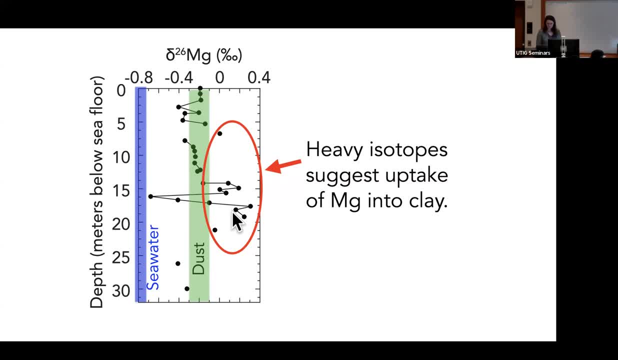 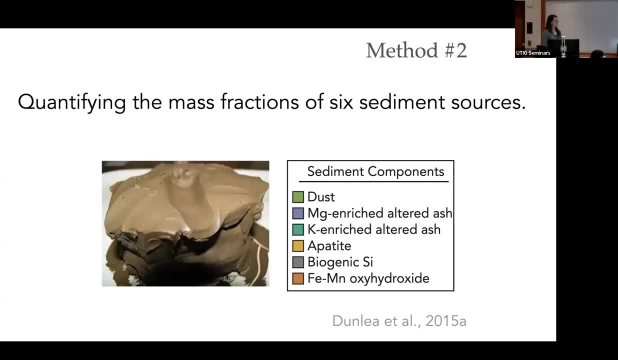 Is taking up, potentially taking up, magnesium. Now this tells us like Okay, we probably have magnesium uptake into clay, but like how much? we can't really use this to quantify the magnitude of magnesium taken up. so for that we turn to our second method, which is quantifying the mass fraction of six sediment sources into the clay. 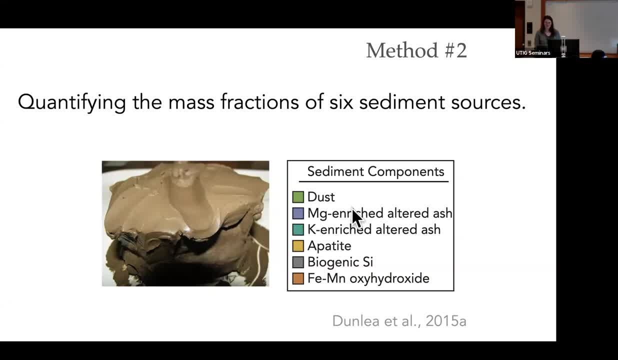 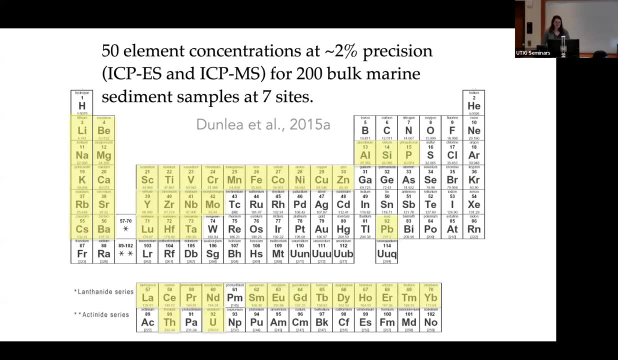 So we're going to take this Brown, homogenous looking clay and tell you how what percentage of each of these end members is in this clay. So these are all the components that mixed to make this and i'll get more into them later. But our first step is to analyze the sediment. like I said, using inductively coupled plasma emission spectrometry or inductively coupled mass spectrometry, we analyze 50 element concentrations at about 2% precision. 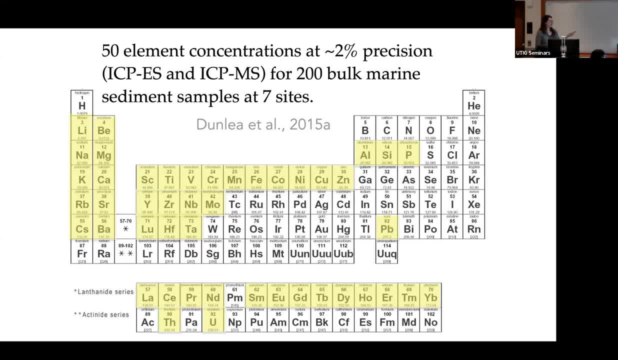 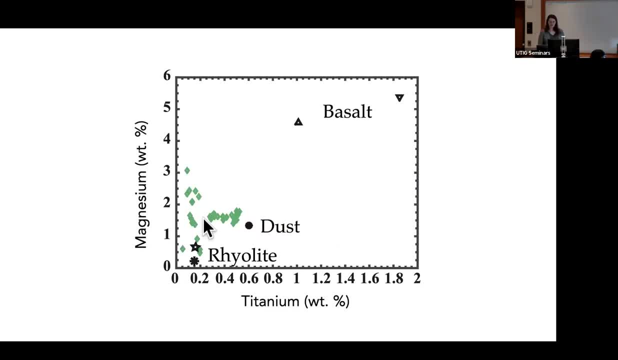 For about 200 samples at the seven sites. The elements we analyze are highlighted in yellow And if we just look at two elements for now, on the X axis we have titanium concentrations, on the y axis we have magnesium concentrations. These black symbols are reference materials. so like average assault, I think this is a mid ocean Ridge basalt and an average ocean island salt. they should plot up here. 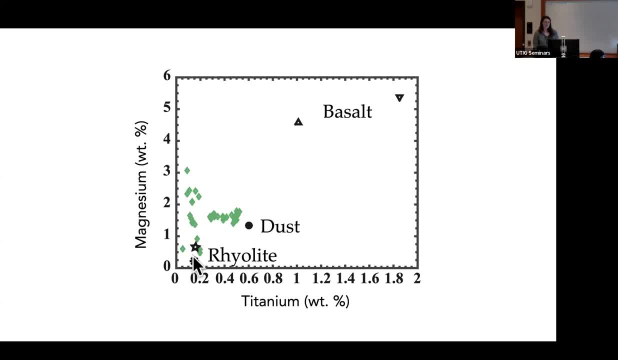 Average kind of material plot around here, and a realistic Or more felsic volcanic ash would plot around here. And if our samples were a mixture of just the salt being diluted by other components that were not aluminum silicate, they should plot along this line. 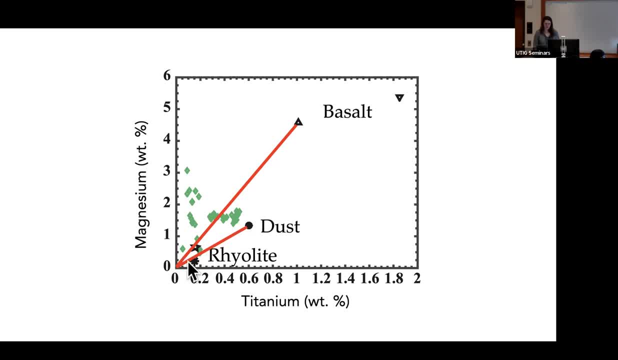 If they were dust being diluted by, let's say, calcium carbonates or another component, they should plot on this line and if they're a mixture, they should plot in between these two red lines. I should also state the green symbols are from our site 1366, and you can see that there's a big enrichment and magnesium. 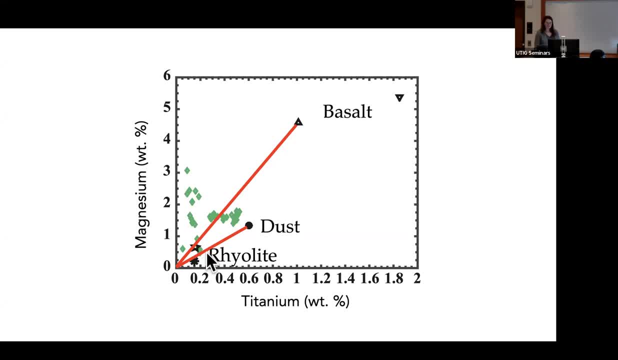 That can't be explained by any of these and members that you typically find in the ocean. so this is a- not our first hint that like, maybe there is a lot of magnesium being taken up into the sediment that can't be explained by detrital sources. 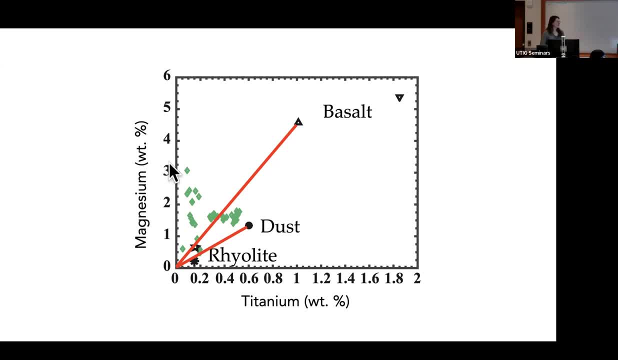 But again, it's from this plot. it's like a little hard to tell like how much. Oh, we did analyze there were some like altered volcanic ash layers and this was one of those layers That we're going to call a magnesium enriched ash or magnesium ash, and it did. could serve as an end member to explain this. 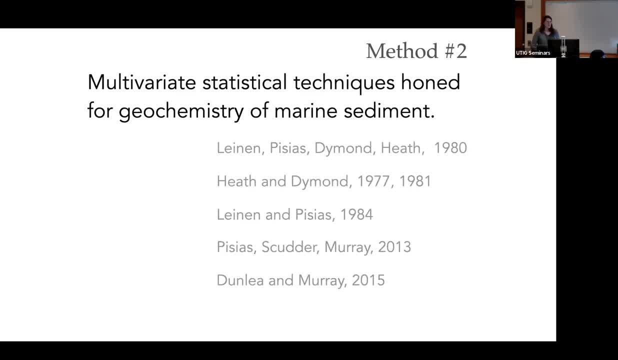 The samples over here. So to quantify how much magnesium is taken out and to kind of look at the holistic picture of what's happening in these sentiments, we did a variety of multivariate statistical techniques that were specifically honed for the geochemistry of marine sediment. so 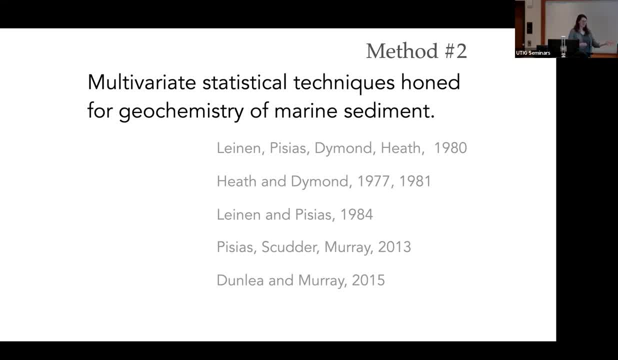 line, emphasize diamond Keith and they're like, have developed these codes over time. My, my PhD advisor, Rick Murray, did his postdoc with Margaret line and and then brought the statistics into his group and now i've been carrying the torch to continue the use of these techniques. 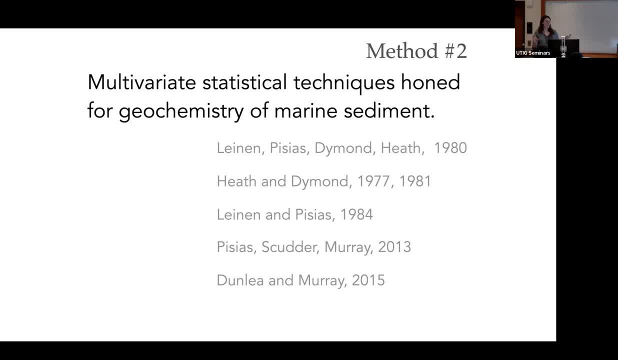 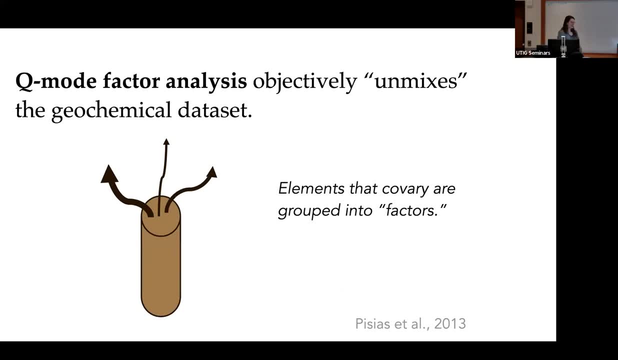 they've been extremely helpful for these types of sentiment where it's hard to pull apart different sources when it all looks the same. So the first technique we're going to talk about is human factor analysis, And Q-mode factor analysis is beautiful because you just give it a data set and it 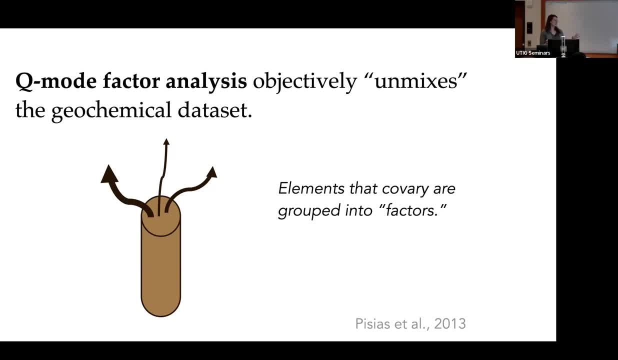 objectively identifies how many components and what kind of components it can statistically differentiate. So we call this an objective unmixing of a data set, And what it's doing is looking at how elements co-vary throughout the samples and then it groups the elements. 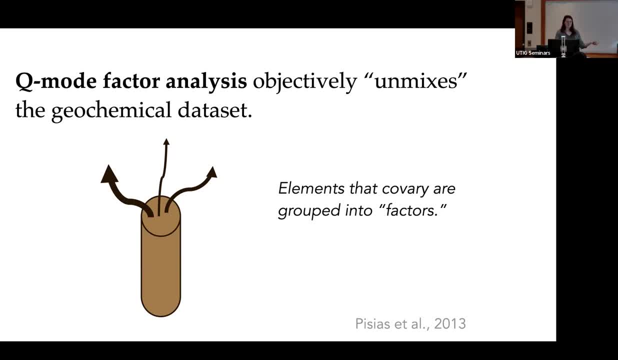 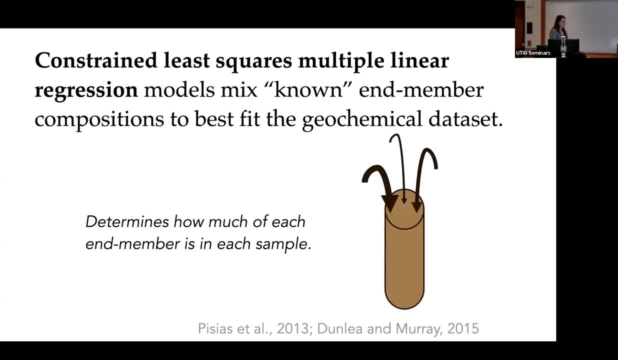 into factors which we can interpret as N-members. So this was the first step we did and it helped us recognize, like how many sediment components we should be looking for and the approximate composition. Then we took that information and found known published values in the literature. 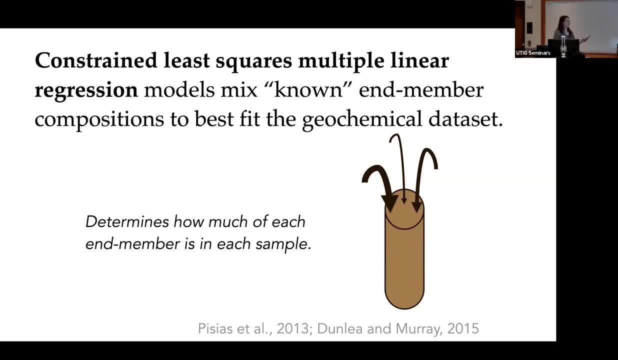 of different N-members and put that in a constrained least square multiple in your regression model. where this one, you take the known N-members and you try and re-evaluate them. And then you take the known N-members and you try and re-evaluate them. 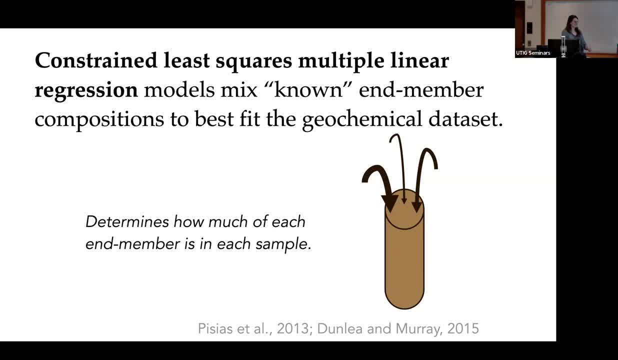 And then you take the known N-members and you try and re-mix them in various proportions to recreate your data set, And so you're trying to minimize the difference between your model and the measured data set by mixing known N-members, And this technique determines how much of each. 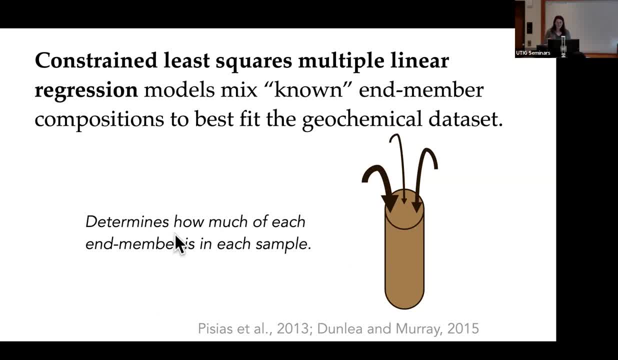 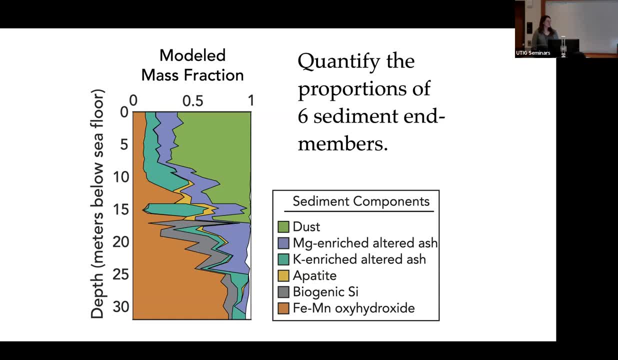 N-member is in each sample, And so that is where we can get a quantitative mass fraction of each of these N-members in the sample. So these are the results from a whole lot of modeling and sensitivity testing and robustness testing, And so what we're doing is we're going to 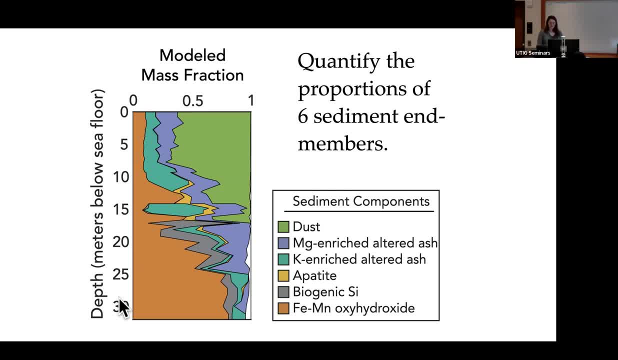 So here in this plot we again have depth in meters below seafloor And on the x-axis we have the model mass fraction. So 0% of the sediment is here, 100% of the sediment is here, And then each. 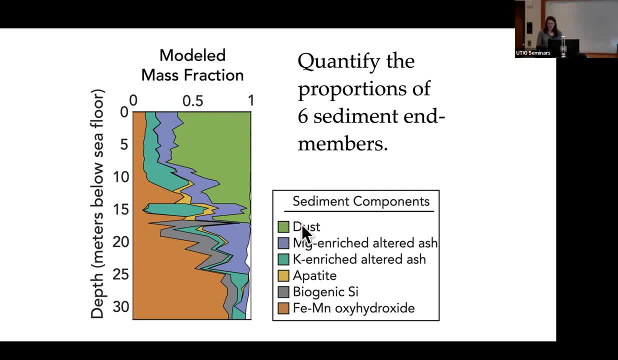 sample is broken down into these various components. So each of these components tells a very interesting story. Dust: we can look at how dust fluxes have changed to the South Pacific gyre over time. This orange part: this is a big hydrothermal sequence that was deposited on top of the basalt. 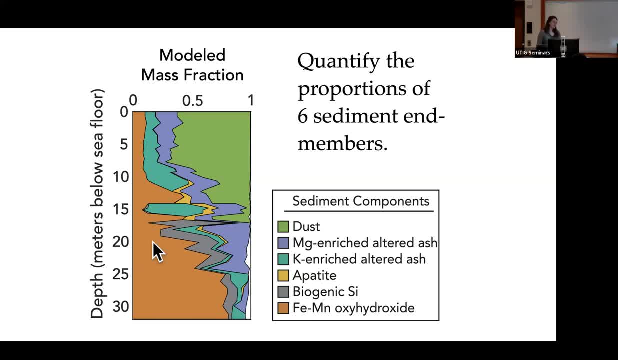 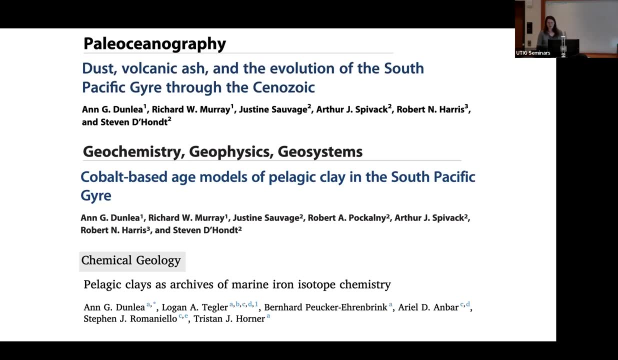 So I have other work, looking more at the metal cycling in this region and looking at this metal, the metal oxides in this component. But today, oh, and all of this like metal cycling and dust stuff, you can read about in other publications, But today for this talk, 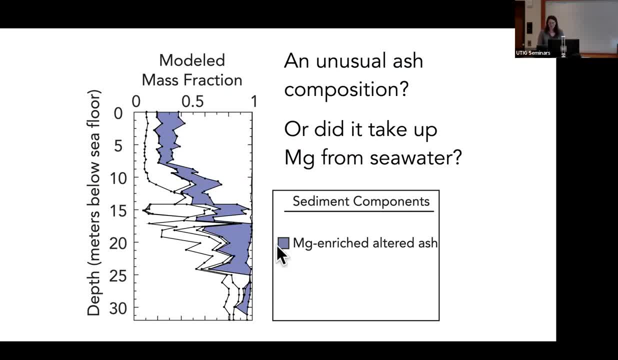 I want to focus on this purple, the purple component, which is that magnesium-enriched altered ash that we saw in the two-dimensional plot. I tried hundreds of thousands, thousands and thousands of models and this end member consistently came up as being a very important part of this sediment. 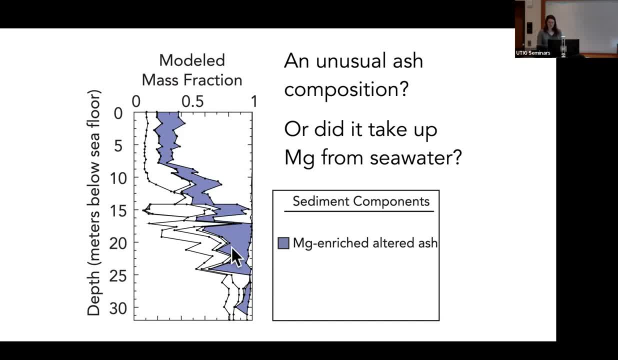 And you can see it's almost in every sediment that this is a thing. So this is the mass fraction of magnesium-enriched altered ash. So this is the mass fraction of magnesium-enriched altered ash. So this is the mass fraction of magnesium-enriched altered ash. 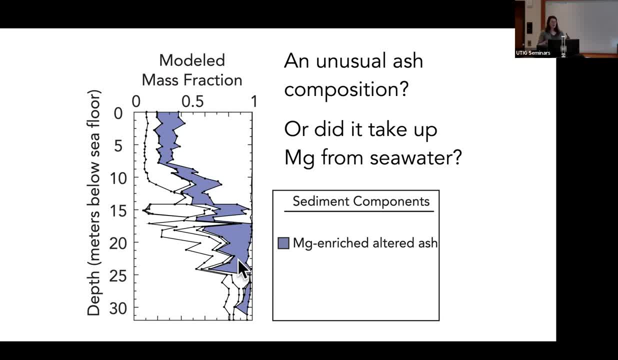 Okay, so this- this end member- we know has like enriched magnesium and we can like quantify how much should be in the ash because we like it broadly. the elements that don't change would suggest it's a rhyolite, So we have an idea of like how much magnesium should be. 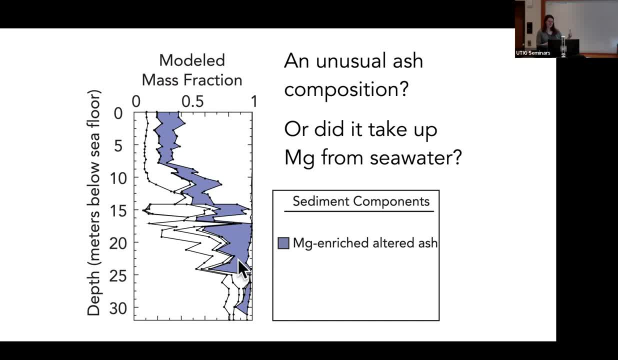 there and then we can calculate how much extra magnesium is there. So we can like quantify how much excess magnesium is there, But can we like really show that that was well, but yeah anyways, so this also suggests it. So let's compare this to our first method. So on this plot, on the x-axis, we have that data. 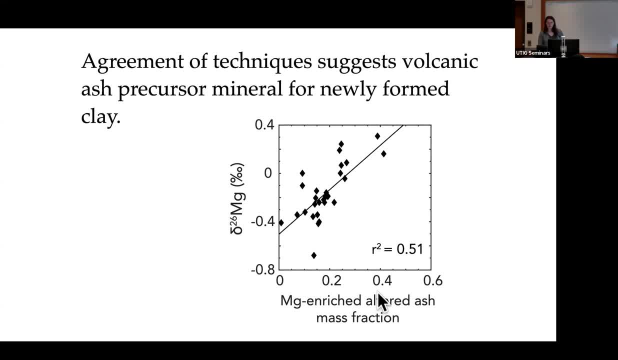 from the previous slide, the magnesium-enriched altered ash mass fraction. We're plotting it against the magnesium isotopes from the first method And, although not perfect, it is a significant correlation between these two techniques. So as more of this magnesium ash fraction is in the samples, you have a heavier magnesium isotope. 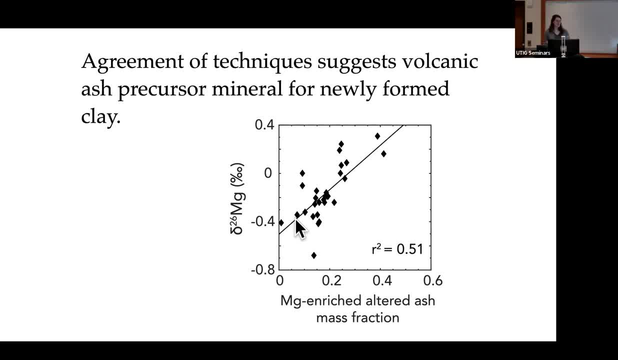 suggesting that that enrichment of magnesium into this ash is corresponding with the heavier magnesium isotopes that we already kind of thought were from seawater, And so the agreement of these techniques suggests that the volcanic ash precursor mineral did take up magnesium from seawater and formed a new clay. 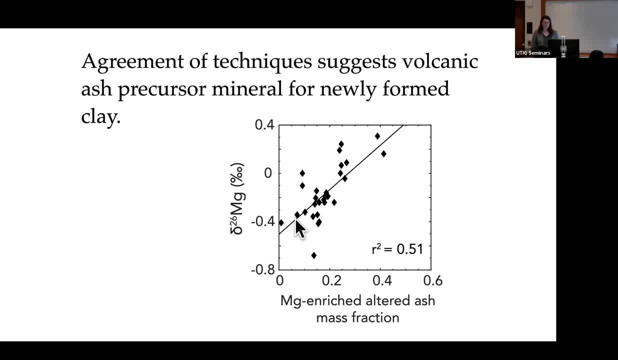 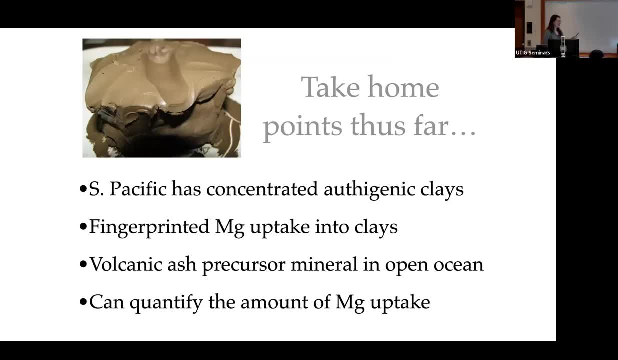 So it's a very significant correlation, Very solid evidence that magnesium is being taken up into at least these segments. So so far, the take-home points are that the South Pacific dryer has concentrated orthogenic clays which are a great asset for looking at orthogenic processes. 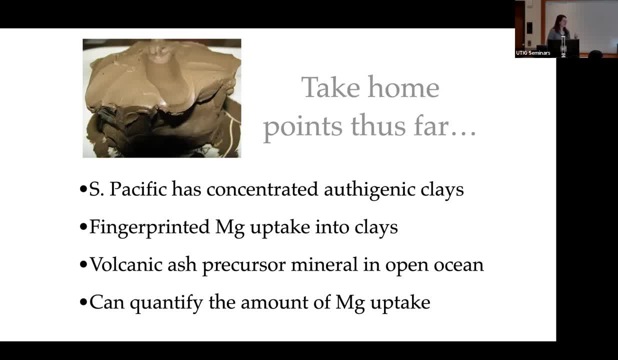 We are able to fingerprint magnesium uptake into clays using the isotopes and identify it as a volcanic ash precursor mineral in the open ocean using the other elements, And quantify the amount of magnesium taken up with all of the modeling work. So we're like, okay, we found some orthogenic clays. How big is this on like a global scale? 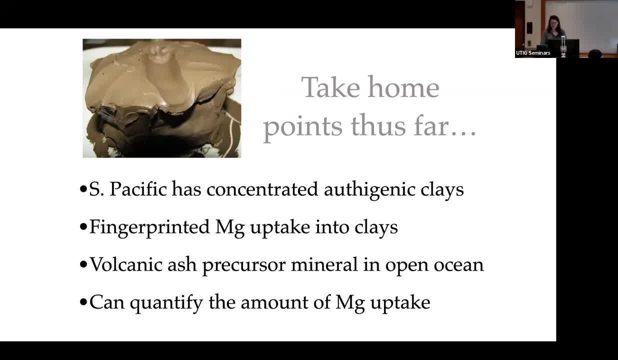 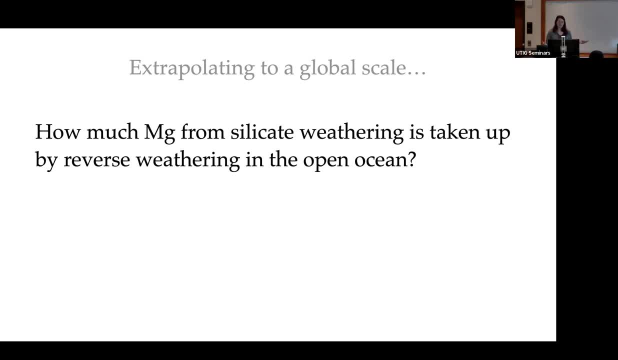 So we took our core top samples, or near modern samples, and extrapolated it to a global scale. So clays are the predominant lithology for like 30 to 50 percent of the ocean floor. They're all over the place. So we were like, oh, this has got to be huge, right. 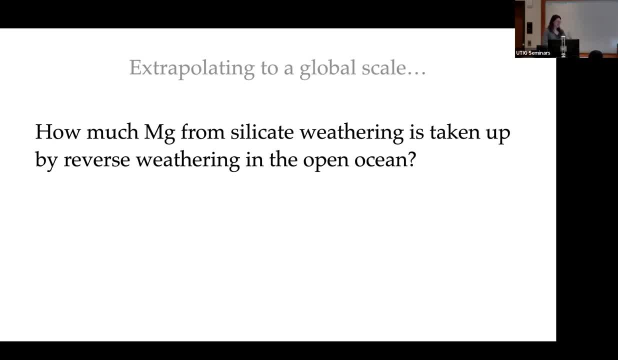 It's, it's. you know, we did all the density corrections and, like our concentrations and how much magnesium we knew was taken up, you know, expanded it to the globe and found that it accounts for 1% of the magnesium coming into the ocean, which, like 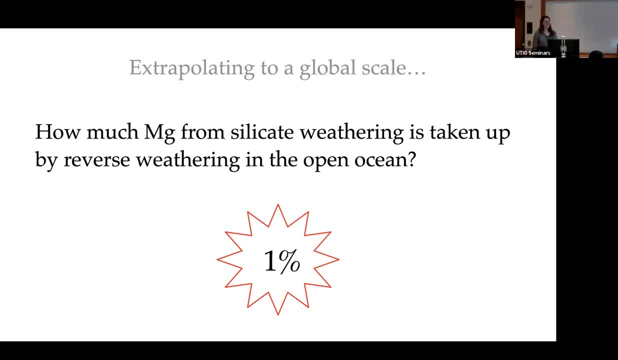 regardless of how you tweak the levers, like it wasn't big, And so I was kind of like, oh, that's disappointing, but not disappointing, You'll learn something. This, this is for the open ocean. There has been other work looking at reverse weathering along the continental margins. 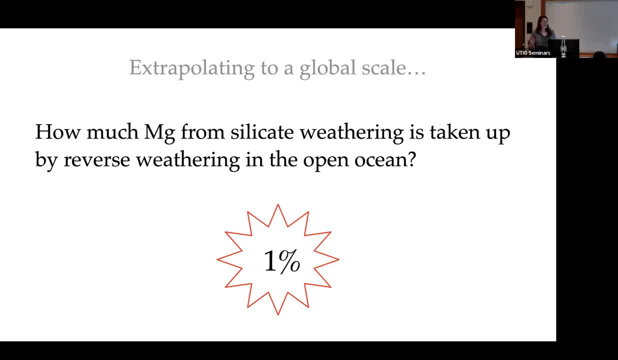 or like right where rivers come out, where you also have a lot of silica And they could, you could have a lot more reverse weathering right along the coastline. So this number is only for the open ocean And we're like, okay, well, maybe more of it's happening near the coast. 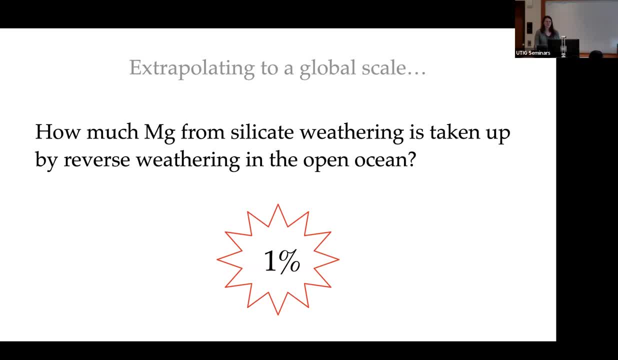 But then we were. we were looking at our data and thinking about the silica pattern And I mentioned earlier that silica in today's ocean is under saturated with respect to silica, So a lot of the ocean doesn't have a lot of the ocean floor did not have excess silica. 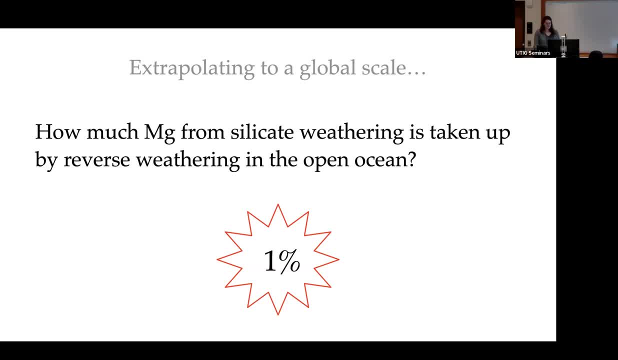 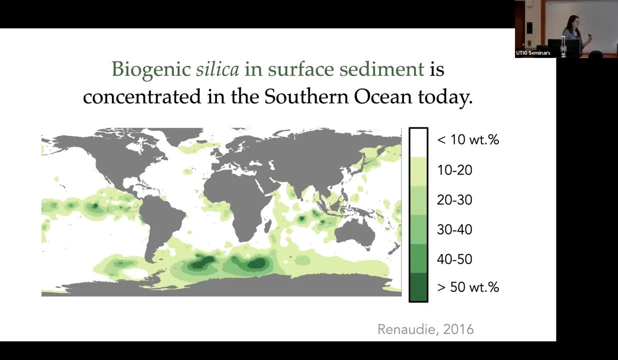 but in the past it was different. So this is today's biogenic silica concentrations in the surface sediment And you can see that the darker green means it has more silica on the seafloor. So the Southern ocean plenty of silica here. 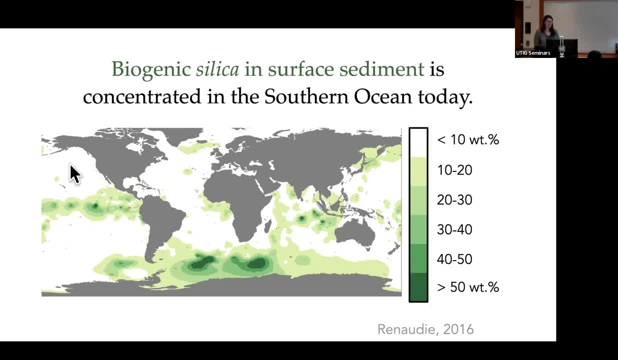 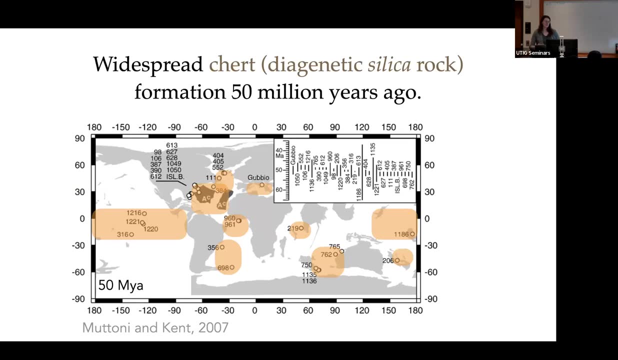 Probably enough silica, but most of the gyres have no silica, And so this is the distribution of silica on the seafloor today. In the past, so 50 million years ago, there has been chert deposited. There's chert that's been discovered from these older yeah, that were deposited 15 million years ago. 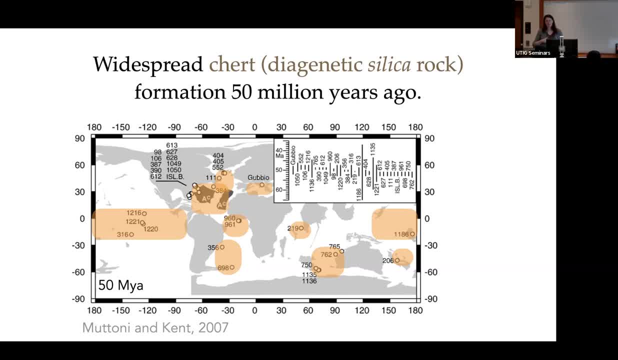 So chert is a diagenetic silica rock, So it is after your body. your biogenic silica goes through a series of alteration products. you get chert, but broadly, if there's chert there was silica is all that we really need to know for this, and almost there's. 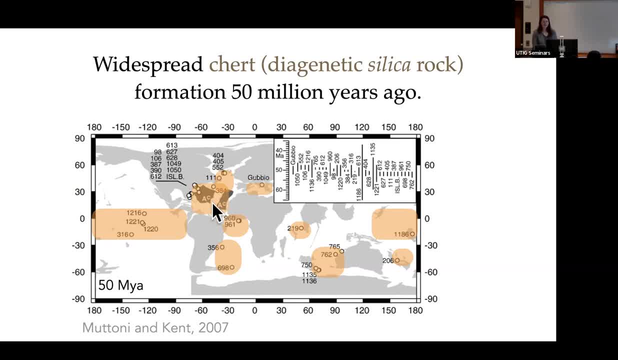 huge swaths of the north atlantic that were covered in, that have been covered in chert and dated to be around 50 million years ago and um, broad bands in the pacific ocean and uh, just chert from 50 million years ago is identified in many, many ocean basins, suggesting that the 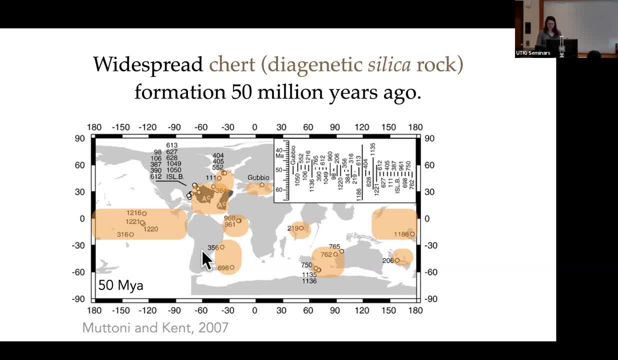 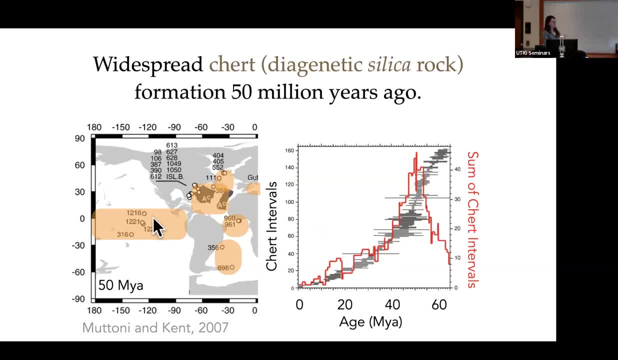 distribution of silica was very different 50 million years ago. and the study by mutoni and kent that was looking at all these chert layers they tried to accommodate for all the spatial biases and and whatever, and stacked up, uh, all of the chert layers they found. so this is aging. 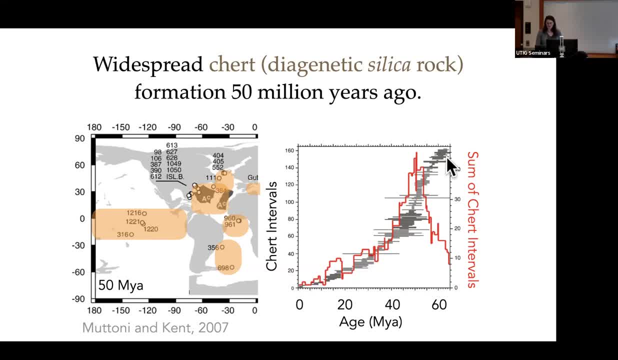 millions of years ago and this is like the number of chert intervals. in gray and then red is the sum of chert intervals, which you know could be adjusted by based on statistics, but broadly they found that the most chert was deposited 50 million years ago. there's a lot of chert layers from 50 million years ago and then 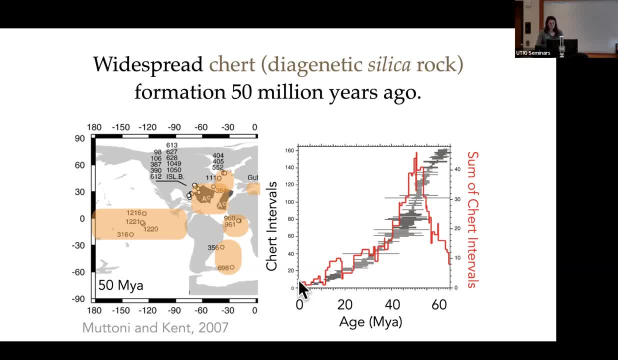 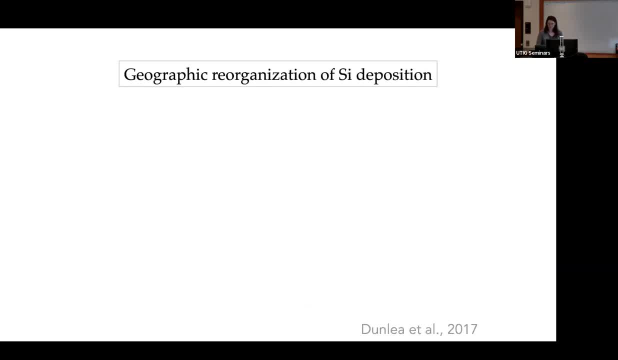 after that it decreased. so this- just this- suggests a dramatic reorganization of the silica cycle from 50 million years ago to today. so if we're going to reorganize the geographic distribution of silica on the seafloor, uh, we're going to have to do a lot of work on the seafloor. 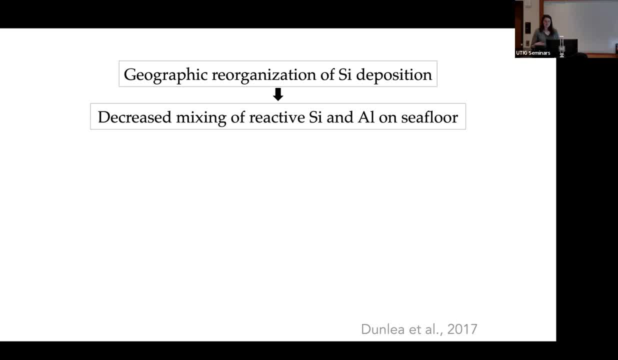 that is going to decrease the mixing of reactive silica and aluminum on the seafloor. so let's say 50 million years ago we had silica everywhere, very easy to mix with aluminum and all the other metals and make new clays over the cenozoic. everything got concentrated into the 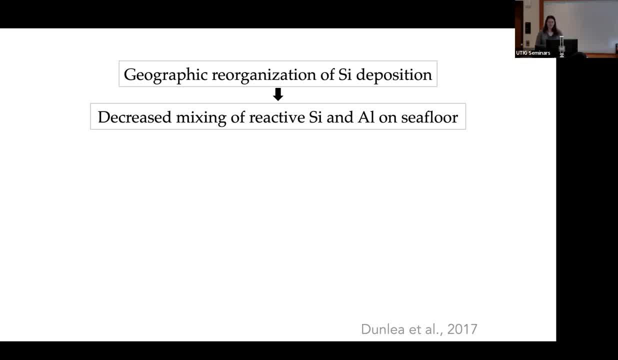 southern ocean or the equator, civic or high latitudes, uh, which that concentration, kind of moving it all down to the southern ocean, stopped as much mixing of reactive silica and aluminum. so this could have, this separation could have reduced the global formation of Othogenic clays. 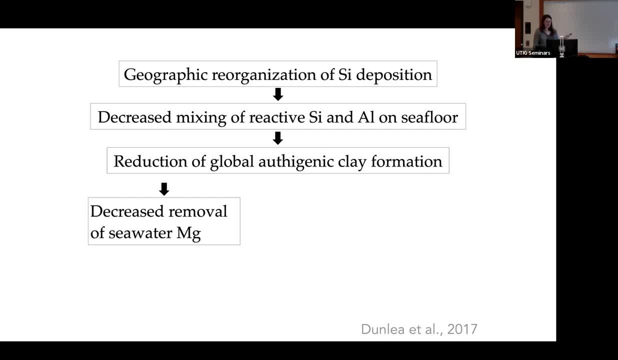 which, if we're reducing the clay sink, we're going to decrease the removal of seawater magnesium, which could potentially increase seawater magnesium calcium ratios, and we took a sample that was farther back that had more Othogenic clay minerals. that would be more representative. it's there's like porcelainite in it in the in these samples from um interesting in our site. 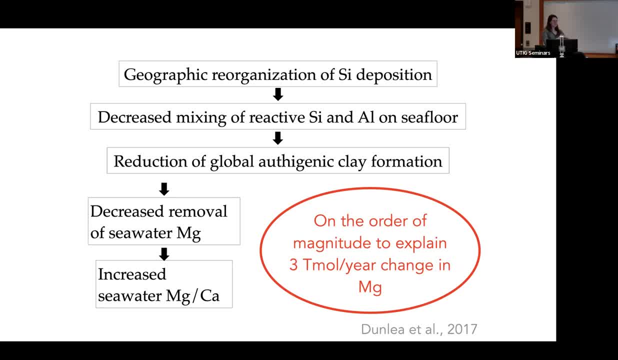 there's silica rich intervals, took the data from that and extrapolated that across the regions of the ocean that we thought would have chert or um like silica, being deposited on the seafloor and staying there, preserved on the seafloor too, and when we did that extrapolation it was on the 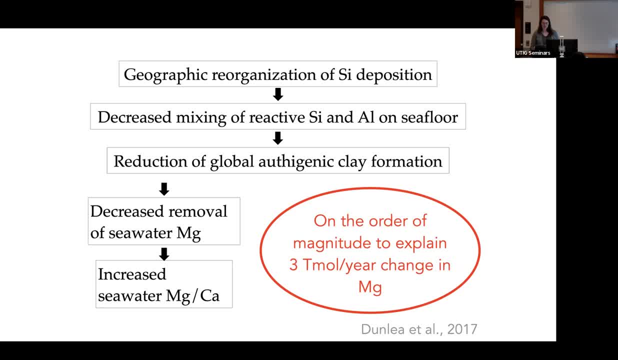 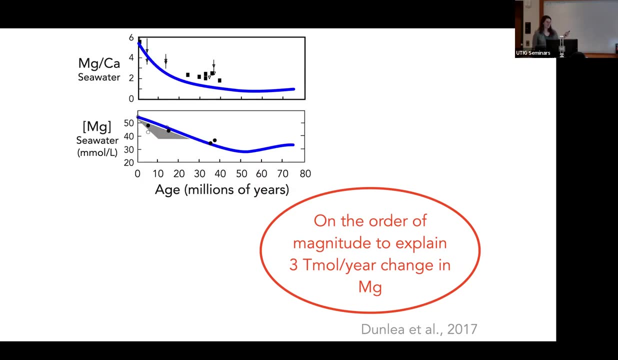 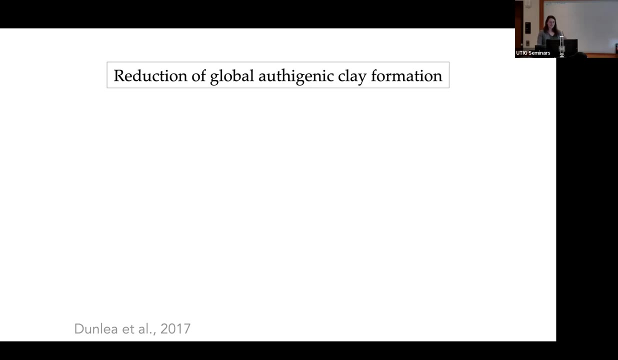 order of magnitude to explain the three teramole per year change in magnesium. so we had one percent of the open ocean today, but potentially enough magnesium uh in the past taking up into these clays. so that might explain these plots. additionally, we have a reduction of global oestrogenic clay formation. 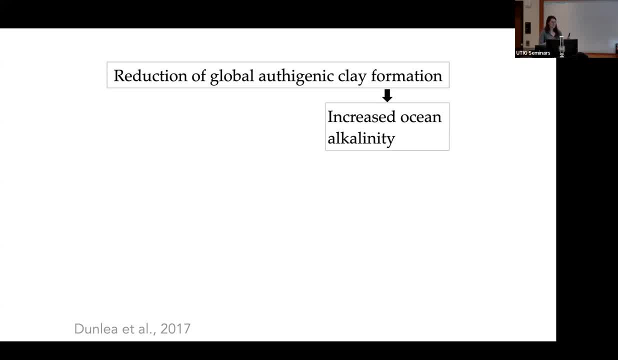 it would cause increased alkalinity because we're not going to be able to use it for the rest of the year. so we're not going to be able to use it for the rest of the year. so we're not going to use it for the rest of the year. 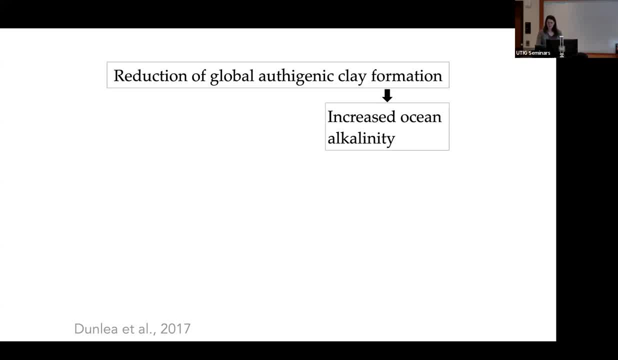 we're not removing, you know, we're not changing that bicarbonate back to co2, and a reduction in that co2 would translate, uh, through equilibrium, to a decrease in atmospheric co2, which would cool the earth and the. and the cool thing about this hypothesis is that, if you 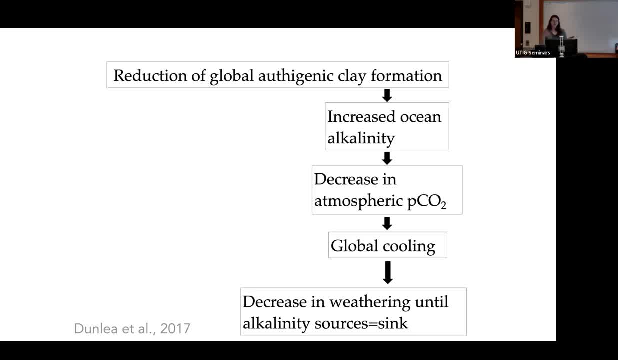 cool the earth like the other ones. we need another system to change to balance and make a new steady state. so if you cool the earth, you're going to have a decrease in atmospheric co2, which would uh, cool the earth. temperature dependent weathering will decrease weathering until the alkalinity. 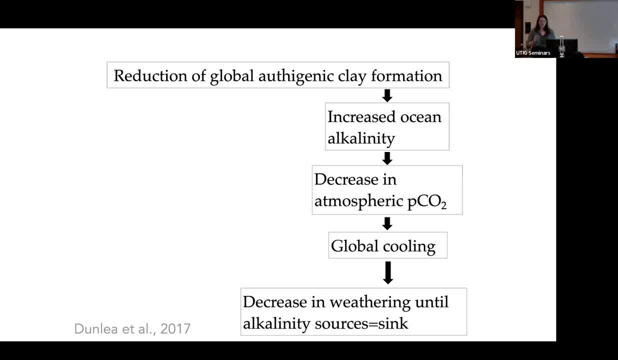 sources equal the sink. so through this way, through the, by saying that a cooling earth will decrease silicate weathering on land, it kind of balances, makes a new steady state by starting with a change in clay formation on the sea floor and if we assume that there's a three terminal per year, 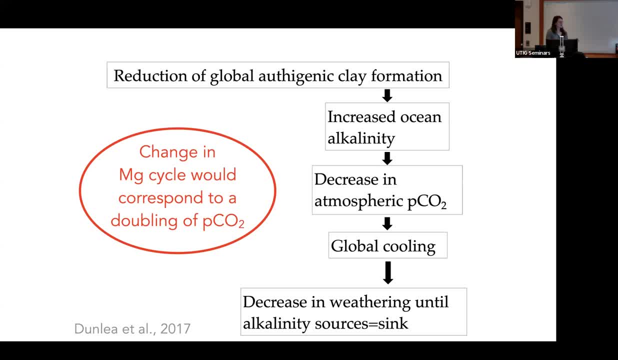 uh, increase in atmospheric co2 will result in ozone and more. when there is a global warming increase in the magnesium cycle, that would translate to a corresponding like doubling of pCO2 from the modern day to 50 million years ago, and that's within a range, I guess. 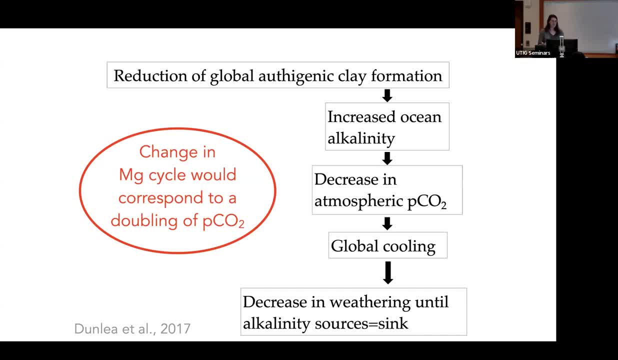 of the wide variety of estimates of atmospheric CO2 that we looked at in that initial plot. So it's within the range that it could be significant enough to explain the CO2.. And so, broadly, just to recap, the ocean floor is starting to change. through this change, 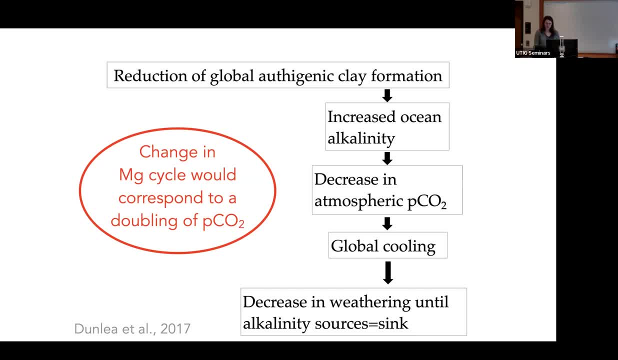 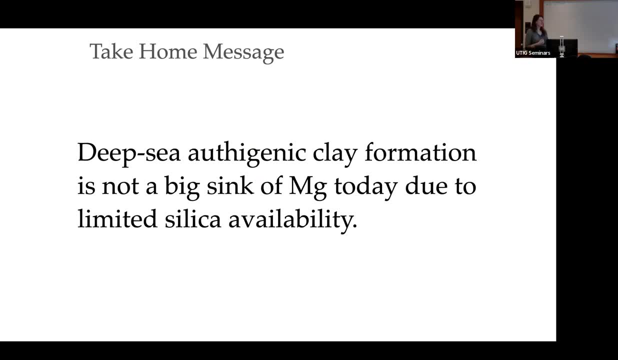 in silica distributions and it's leading to global cooling. So the big take home message here is that deep sea oestrogenic clay formation is not a big sink of magnesium today, probably due to limited silica availability, but it could have been far more. 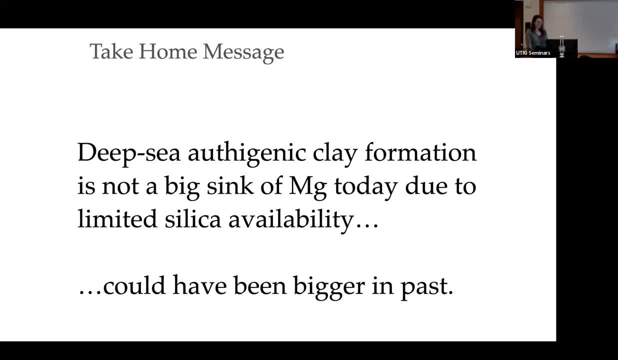 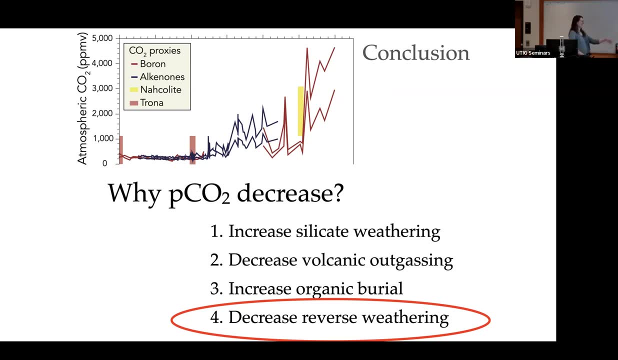 It could have been far bigger in this past, and the change from the past to the present could be responsible for the change in atmospheric CO2.. So I don't think I'm going to claim that this is the only thing happening, but it's a fourth. 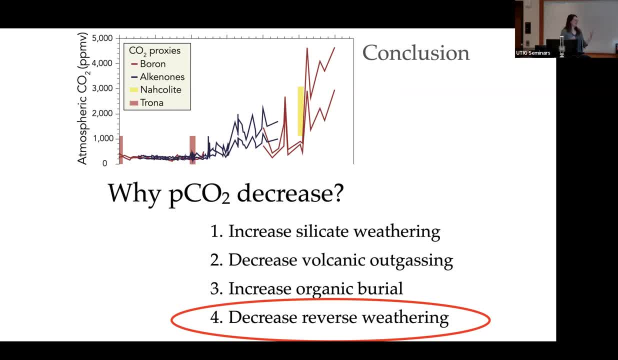 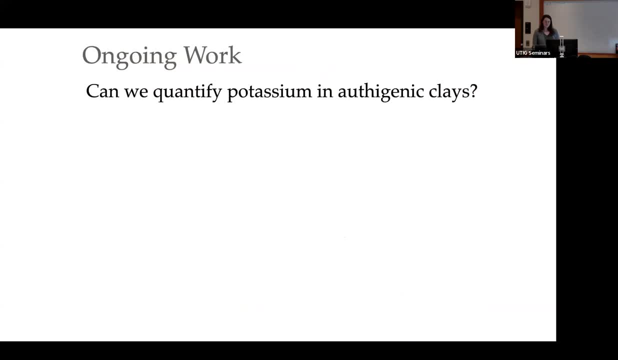 hypothesis, in addition to the three of ways that we could get this atmospheric CO2 decrease, And I guess so that's kind of the conclusion of this hypothesis- ongoing work that has stemmed from this, then projects that I'm involved in include: can we do this for potassium? 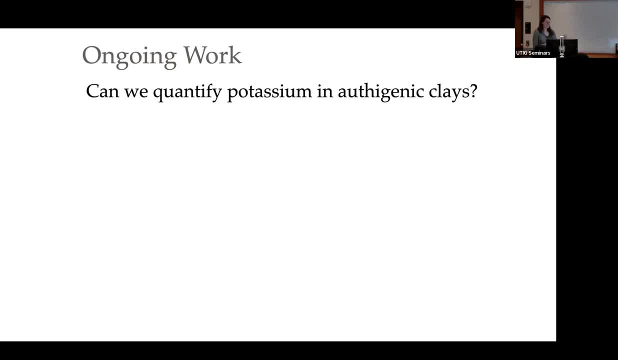 Where's the potassium going? I was hoping it'd be. as you know, I could just do the same thing that I did with magnesium, but it's not that easy. but we're getting there. How do volcanic ash and the carbon cycle interact in different diagenetic environments? 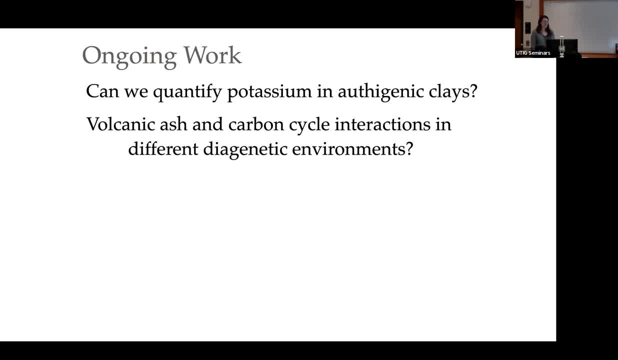 The one in there is a really methodological one. It's not that easy, but we're getting there. How do volcanic ash and the carbon cycle interact in different diagenetic environments? The one in there is a really methodological one. It's not that easy, but we're getting there. 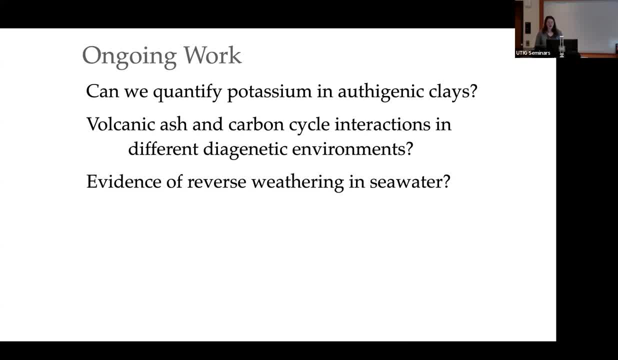 How do volcanic ash and the carbon cycle interact in different diagenetic environments? The one in there is a really methodological one. It's not that easy, but we're getting there. What's happening there between volcanic ash and the carbon cycle? 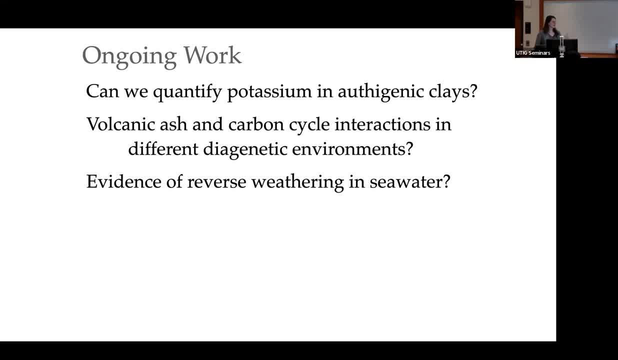 Is there evidence of reverse weathering in sea water? Is there evidence of reverse weathering in sea water? So one of my colleagues that's modeling a seawater carbon cycle is brought to the door there. well, we haven't published this yet, but we'll get there eventually. 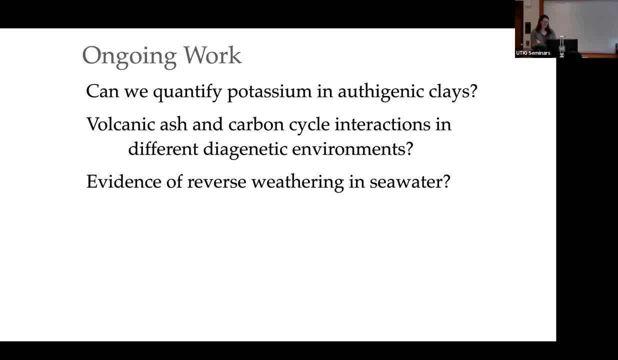 We're looking for evidence of reverse weathering in the carbon cycle coming from a sediment sink, And these oxic marine sediments are a big sink for a lot of different metals, And so there's metal isotopes that are being developed as paleoproxies and being applied to early earth and paleo records without having a great idea of how it works in the modern day. 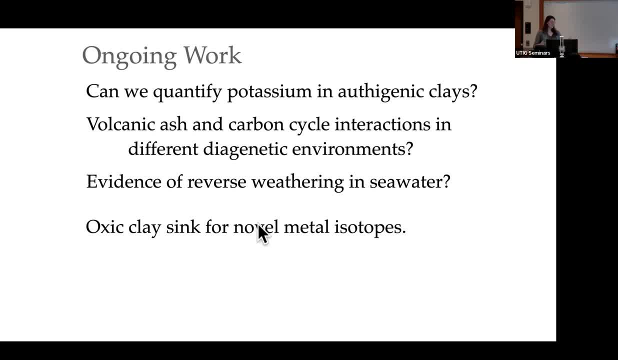 So we've been looking at how these oxic type of clays that cover 30 to 50% of the seafloor and the impact they're having on metal isotopes. I mentioned that big hydrothermal sequence at the bottom of the site and that's led to work looking at the distribution of hydrothermal metal deposition. 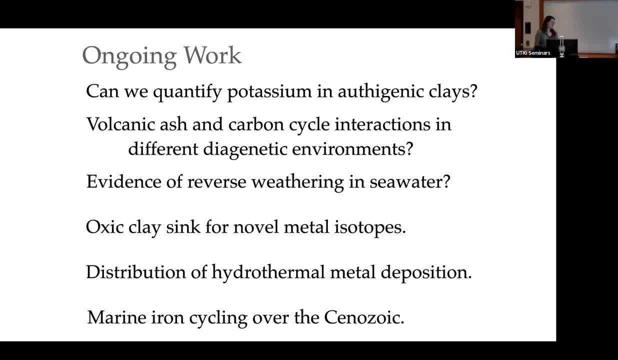 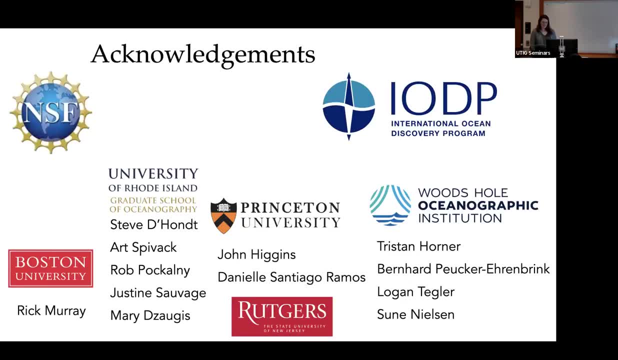 And then also we have one paper out and another one coming out, hopefully soon, about the marine iron cycle and looking at the different sources of iron and how those have changed over time, And with that I would like to acknowledge my PhD work. 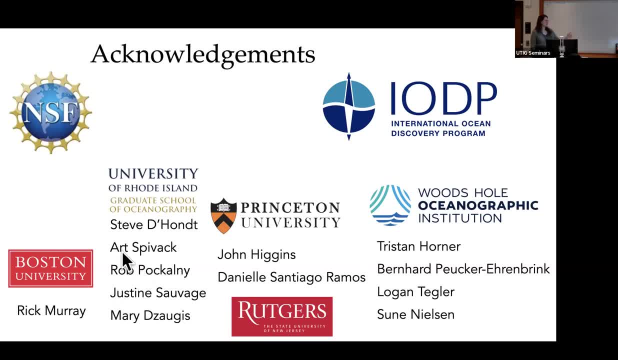 And I. I have done postdoc work with colleagues at Boston University, University of Rhode Island- I guess Rick is now at HOOI, but whatever Princeton University- Danielle is now at Rutgers, who is a co-author on this study, and then my colleagues at Woods Hole that are current collaborators. 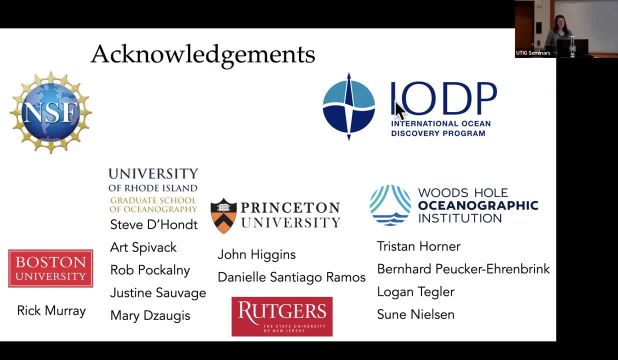 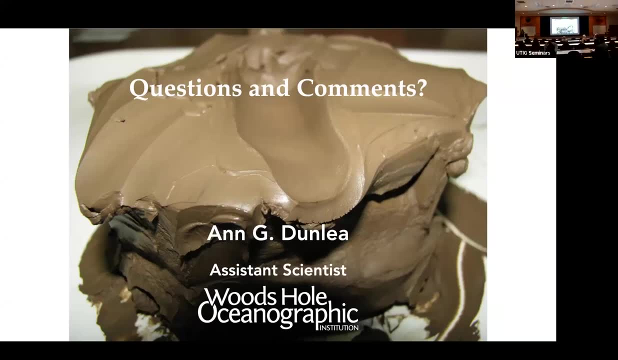 And, of course, none of this would be possible without funding from NSF and none of these samples would exist and all of these records that I showed you today wouldn't exist without the the International Ocean Discovery Program. So, thank you, That was really cool talking. thank you, We have plenty of time for questions. Constantino's: preparing the cube. 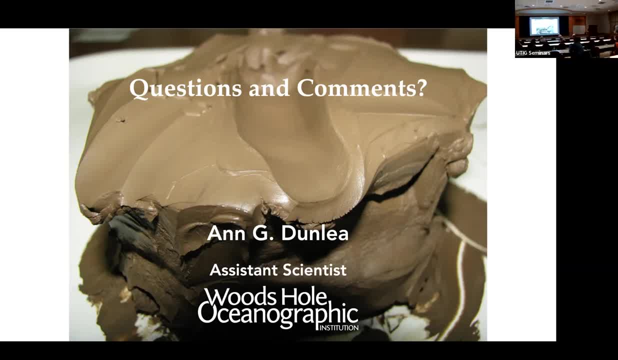 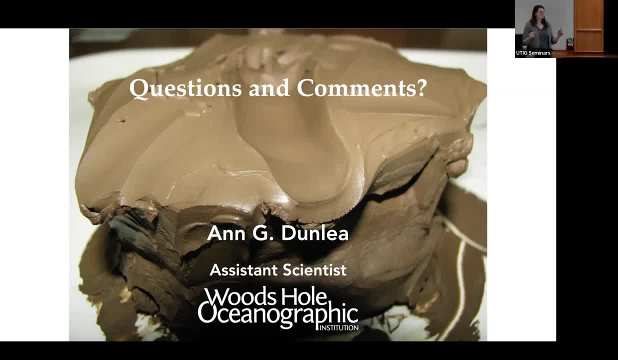 And also like like, yeah, just like silica distribution and In general, and where those like starting with the nutrients and having nutrients be redistributed and then kind of reinforcing itself with the biological changes. so I i'm not sure. but Thanks, it definitely did change, yeah. 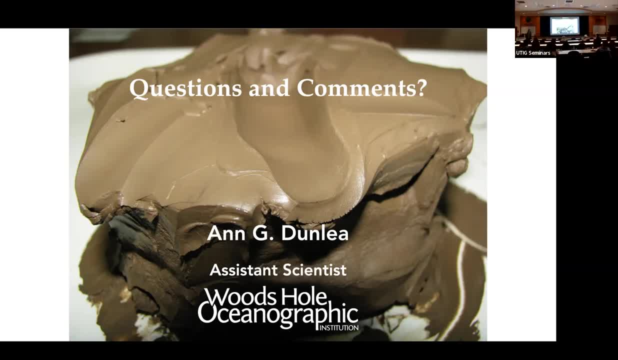 we're in the middle of this global experiment where CO2 is going up again and obviously it's happening very quickly but very recently. is there an element of this you could check Looking at at at modern rates, and could any of this, did any of what you're doing here, apply to looking at very, very recent reactions? 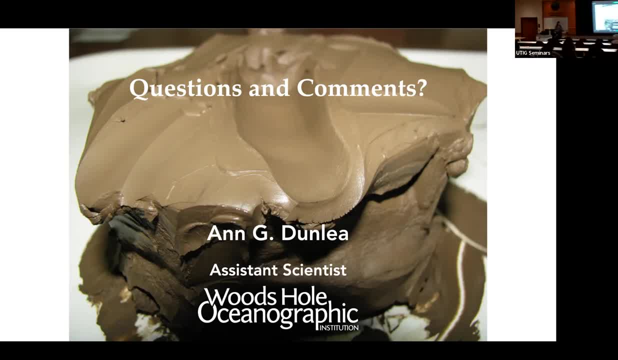 Yes, so a lot of the evidence that kind of like ramped up reverse weathering, it's an idea- was on Amazon, like the Amazon delta, like delta systems, content merchants. So those are all much faster processes and the studies and lab that have tried synthesizing these. 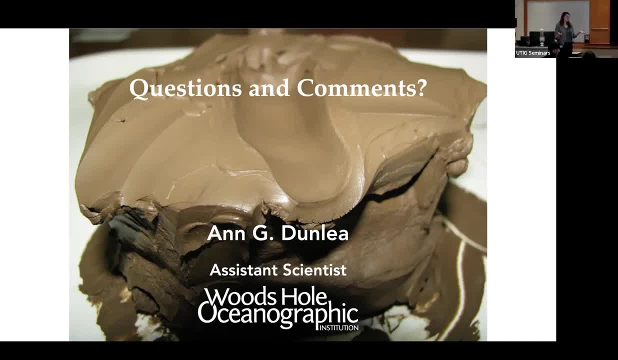 systems, content merchants. so those are all much faster processes and the studies and lab that have tried synthesizing these types of authentic place. it doesn't take very long- it's like weeks, I guess- And so they do. they can potentially have an impact on on more human timescales as well. i've been thinking about this a little bit in terms of like carbon storage techniques, either, like if you're increased weathering on land as a way to remove CO2, like How much reverse weathering happens Once it gets to the ocean, or can we inject CO2 into the seafloor, react with volcanic like and weather volcanic ash, and how much of that is actually weathered versus reverse weathered in that process. so i'm not sure I fully answered your question. 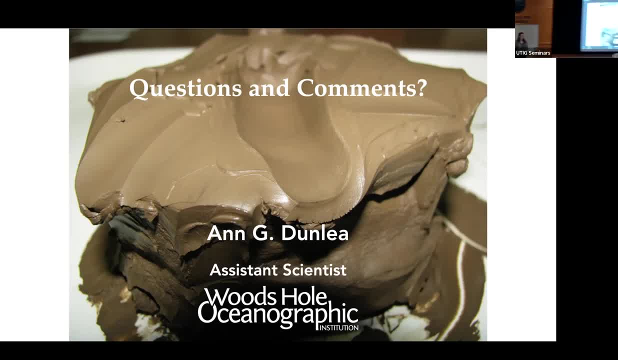 And I don't know, But it strikes me that we're in this major shift right now. it's small relative to across the center zone, but still some of this has got a bear on the planets, responding to big changes In chemistry. Thank you, 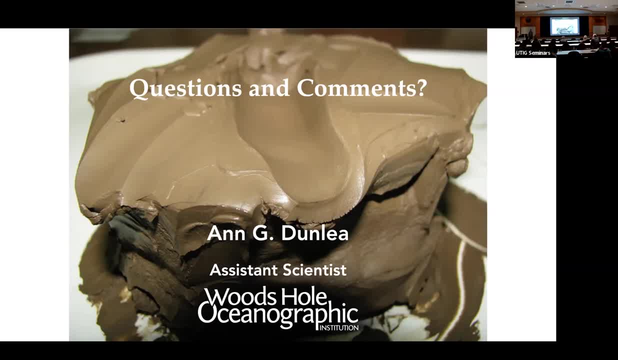 enjoy the talk very much, showing. you mentioned ocean gateways. i'm going to bring that up. it seems like you, by just ignoring them, you sort of dismiss- dismiss the old candidate hypothesis about the opening of the southern gateways. I think they're incredibly important. I didn't mean to seem dismissive. 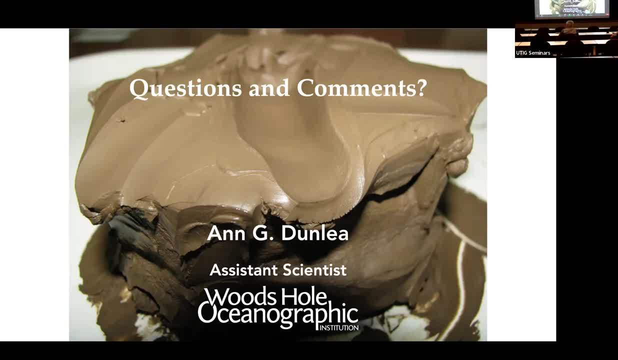 strongly related to that is what, in your view, would cause the rapid decrease in temperature in the myosin. There is a hypothesis about that and it's in the in the good gateway story From the Scotia sea. how would you increase that rate of descent into the ice house? 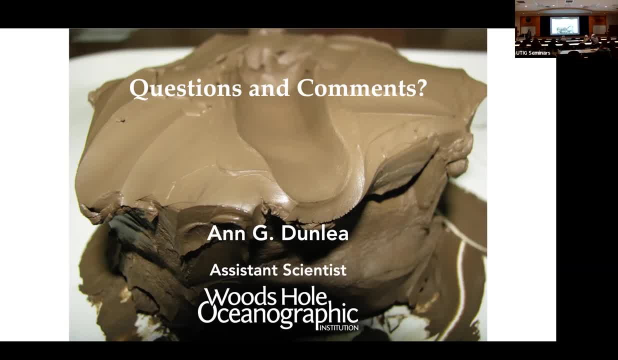 yeah, um, uh, I Okay. well, I did want to reiterate that the, the gateway opening, clearly had significant changes on our ocean chemistry, climate and everything. so I don't think i'm not gonna, i'm not going to dismiss anything. it definitely probably played into it and 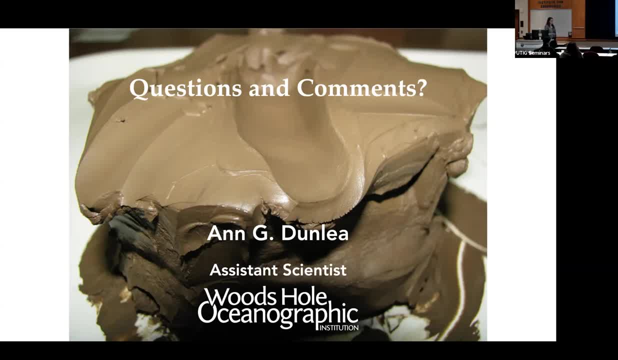 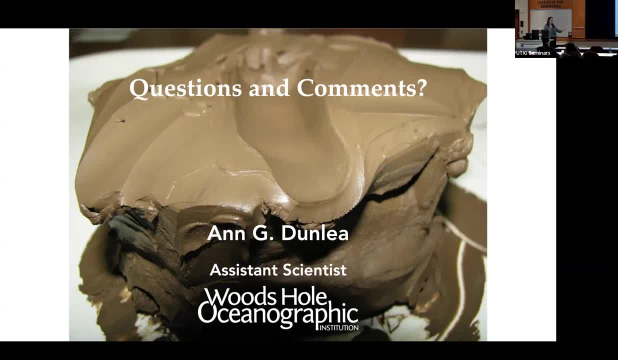 I don't know, I don't. I don't actually dismiss or throw out any of the other ones, i'm just suggesting another one. Thank you, who's good Thanks? thanks for your great talk. i'm still trying to understand the dynamics of the composition of deep spillage of clay. so I understand that these clays, they precipitate. 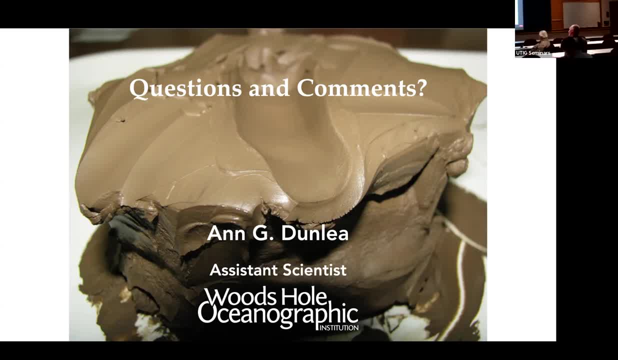 Possibly trigger, for example by by ashes or dust. I was wondering if it also necessarily then binds These, These, These elements such as chlorine, magnesium, potassium, that otherwise would stay dissolved in the oceans. yeah, so the chlorine story I I I know very little about. the potassium story is a little bit more interesting, because we ran potassium isotopes on the same sediment and I was hoping that they would correlate with the other ash that's in there and be like: oh, this one took up magnesium and took up ash. 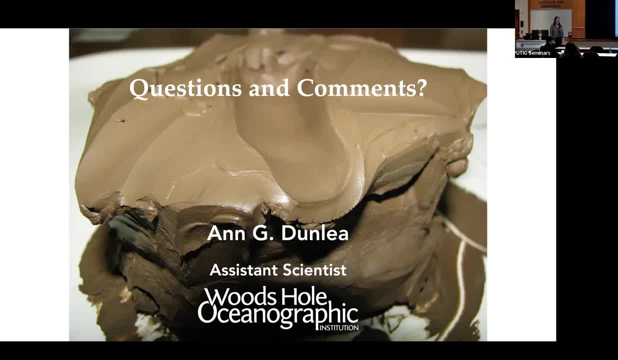 yeah, but there's zero correlation. So that has kind of forced us to look at other scenarios. I think one of the issues with the South Pacific gyro sediment is a lot of the ash is more felsic or like closer to a rye light composition which naturally has a lot of potassium, so an uptake in potassium and already pretty potassium rich sediment. 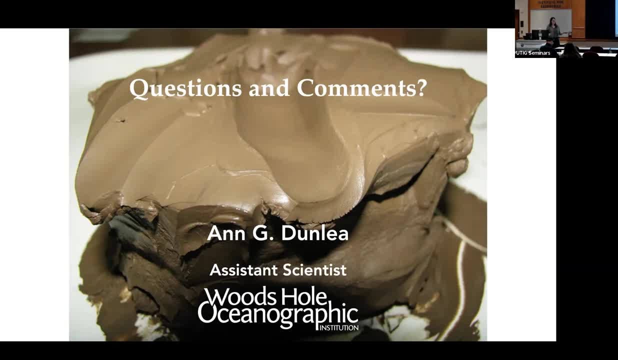 is very challenging. In some of the other ocean sentiment i've been looking at that are less realistic and maybe more anesthetic and stuff you can. In some of the other ocean sentiment I've been looking at that are less realistic and maybe more anesthetic and stuff you can. 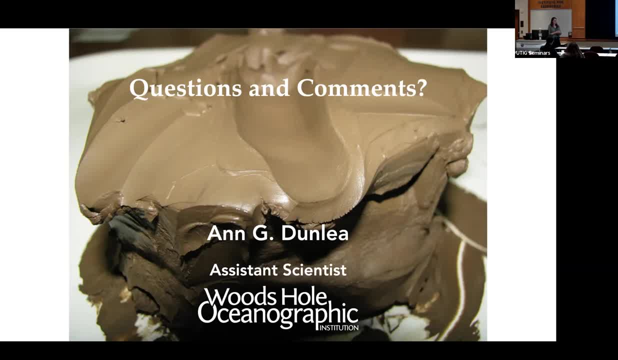 It might be easier to identify our or. they've had a lot of success like looking at this, so my so and the salt, and looking at the weathering or uptake of potassium to assault and tracking that. It has my stuff so can't speak to client, but potassium we're working on. it's not a one for one way of applying the methods. Thank you. 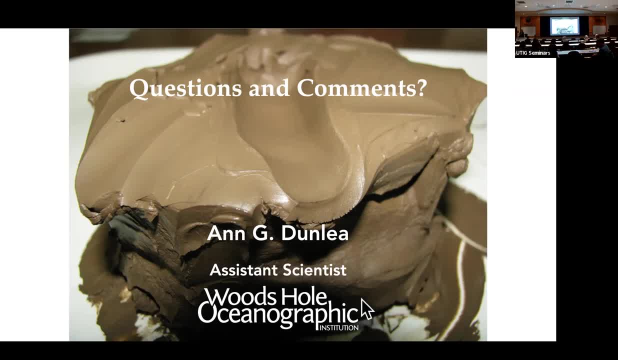 So Benjamin Kiesling asks, or he says, first of all, thank you for your talk and then asks: you mentioned that some of the critical elements in this reverse weathering process come from rivers. I'm wondering what role hemispheric and global scale glaciation might have played in driving. 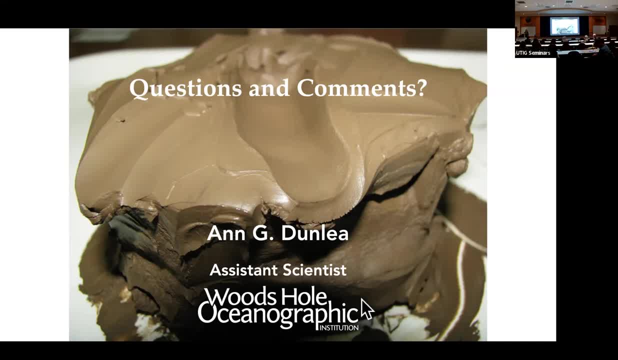 changes to this process. I know dating the sediments is difficult, but so you see any changes in your record associated with known changes in global ice volume and therefore weathering and erosion, for example, the mid-Miocene-Pliocene-Pliocene transition. mid-Pliocene transition, for example. 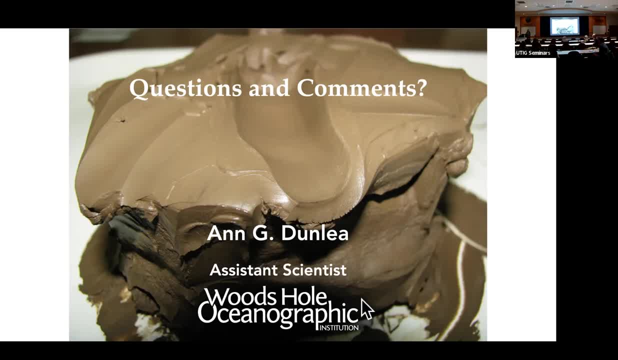 Yeah, great question. So the sediment where I'm talking about- definitely not rivering- It's all windblown or like maybe submarine volcanoes contributed to it, So I can't really speak to the rivering. It's also pretty hard to date like the exact, like boundaries. 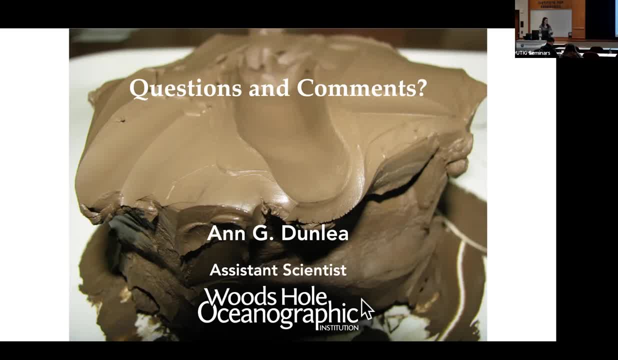 We have done. I've done. We have cobalt models and osmium models to date, these clays and there's like a couple of other age constraints. but it's difficult, like I said at the beginning, these are long records that can cover the whole sentence of us, but you can't really get like here's. 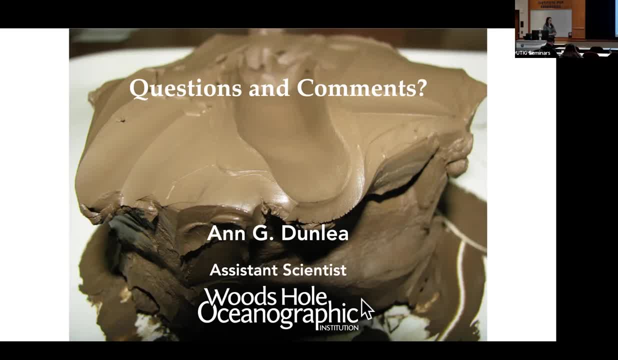 the Miocene boundary. but broadly we can see that that would have to. we would have to look at different sites and kind of do global analyses of, like where the silica is at that time And, yeah, where where it has been. I don't have a great answer for that. 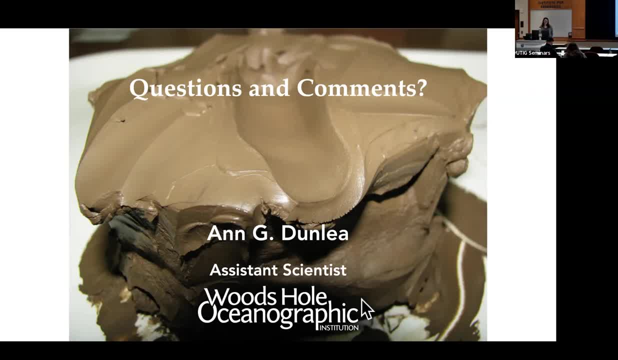 I'm just sort of saying things that are related, Yeah, but it's an interesting topic and I'd love to speak with you more about it. Other online question, And so I was there any August sober. I'm sorry if I messed it up us. 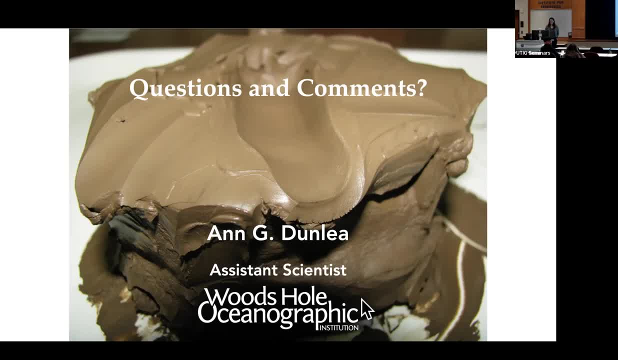 If atmospheric CO2 has been decreasing and still is, then why are we talking about global warming because of increasing CO2? Yeah, Yeah, Yeah. Um. so I think about, like CO2 in the atmosphere, as like like every, all these carbon reservoirs. 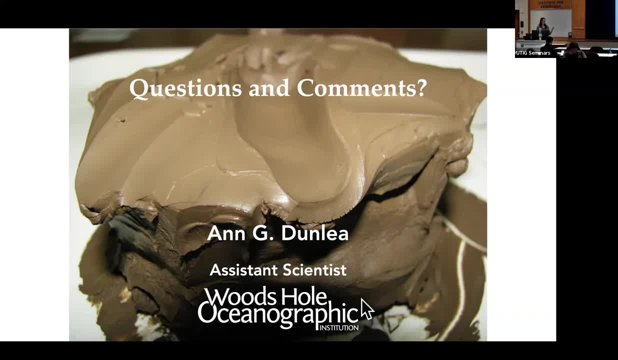 are responding on different time scales And so, like the seafloor, sediment and the ocean are responding way slower than like, like- I don't photosynthesis, or like land, like things, uh, but for the modern increase in co2 we're taking a reservoir, that is. 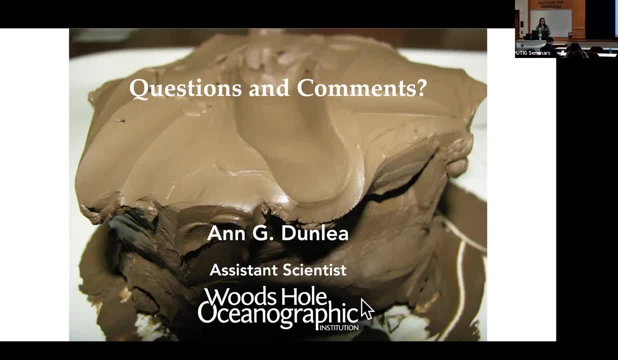 really supposed to be stored long term and making it go quickly into the atmosphere, way more fast than it should be. and so taking something that's supposed to be reacting really slowly with earth and putting into a reservoir that's rapidly reacting, uh, has not been done previously in earth's climate. so, uh, yeah, it's we've. we humans have grown accustomed to living. 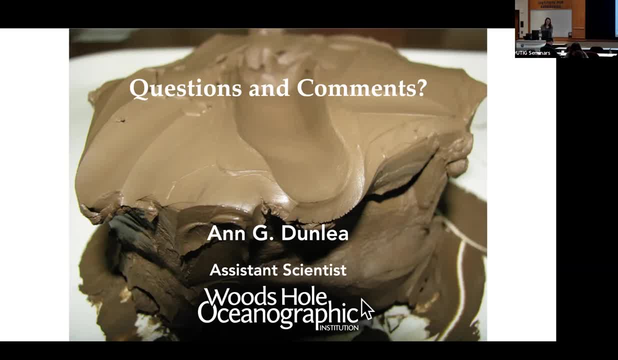 in an ice house world and we're might. we'll probably get out of that soon at this rate. i have a question that's kind of related to benjamin's um. so you said when you were drilling you had this 30 meters, which was really slow accumulation over a 95 million year old. 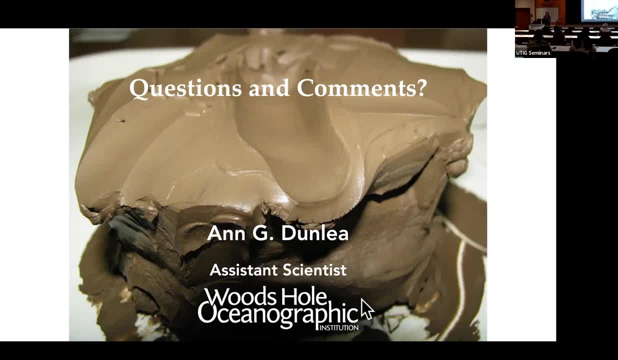 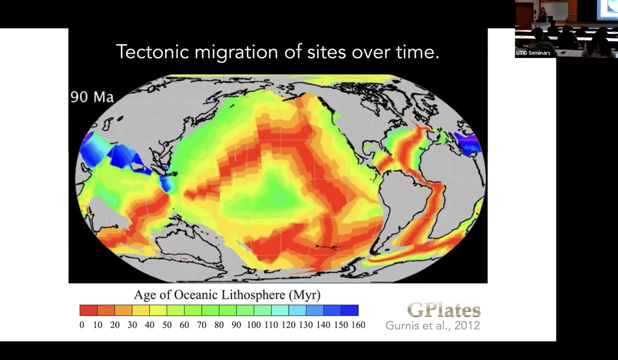 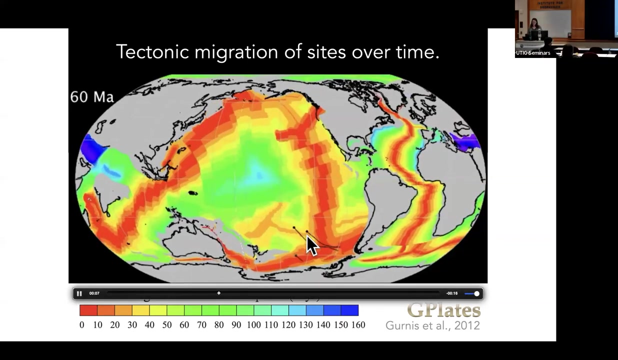 oceanic seafloor. so can you um combine like plate tectonic reconstructions to kind of see like a pathway of where these things might have had like fluxes coming in from? yeah, so, um, there's convenient. you asked, so actually i can point to here. this is the site that we are uh talking about here. so it started. 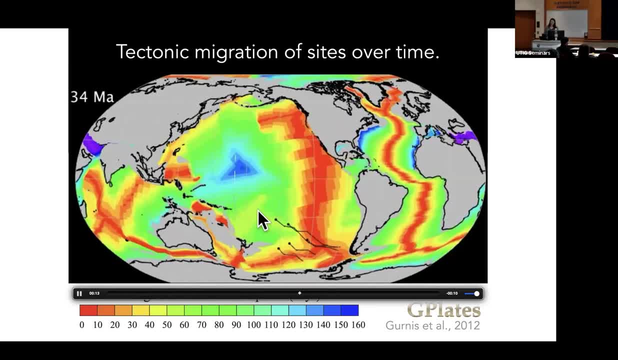 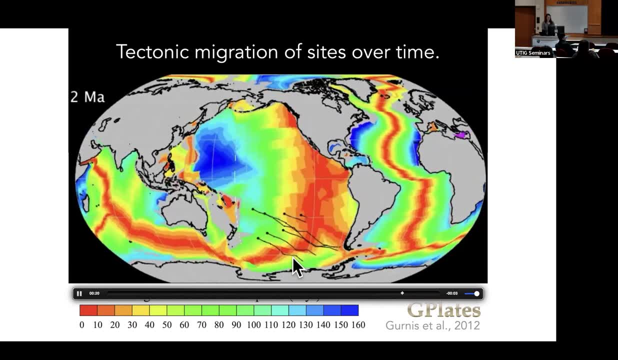 over here when the mid-ocean ridge was farther over, and then it's moved over there. so you can see australia migrating north, south america or migrating more. and the colors are the age of the ocean lithosphere. so the red is the youngest seafloor and the blue and purples are older. 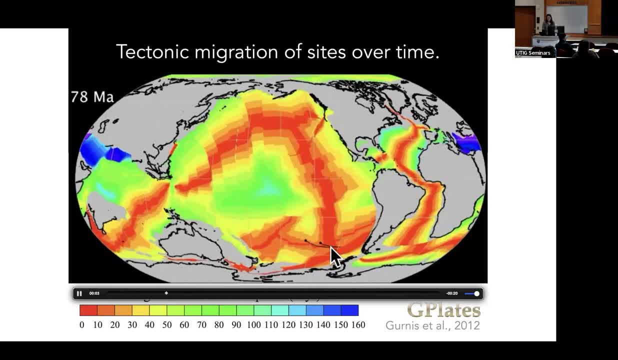 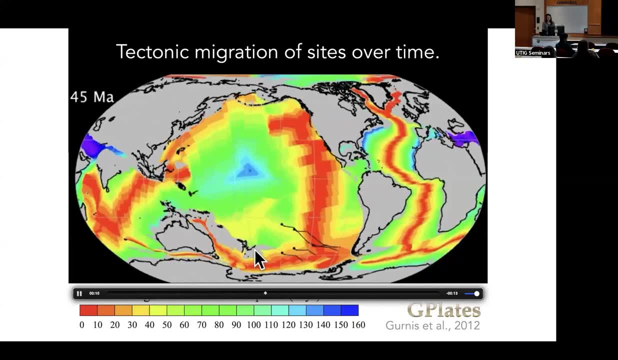 so i started over, so it's born. so so you can kind of. there are studies that try and model ocean circulation 50 million years ago and they have. some of them have like subpar polar gyres there's there's a lot of contention around what the ocean currents are doing. i think 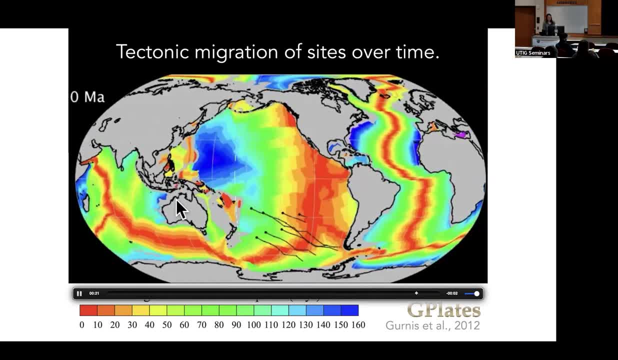 and um, but broadly it's moving that way, so it is getting closer to australia. um, well, that's the whole dust story. but yeah, i can. what was your exact question on this? i mean, yeah, just kind of that, and then i guess you can also see how like the that first section of hydrothermal possible. 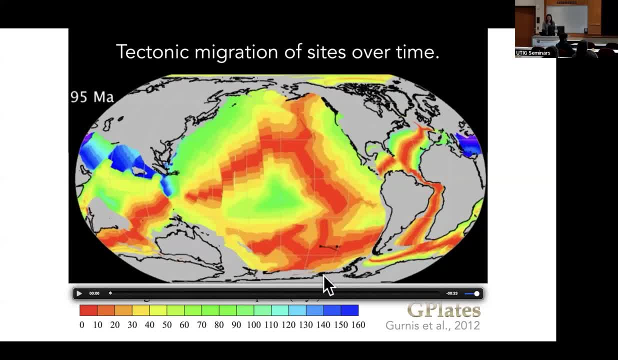 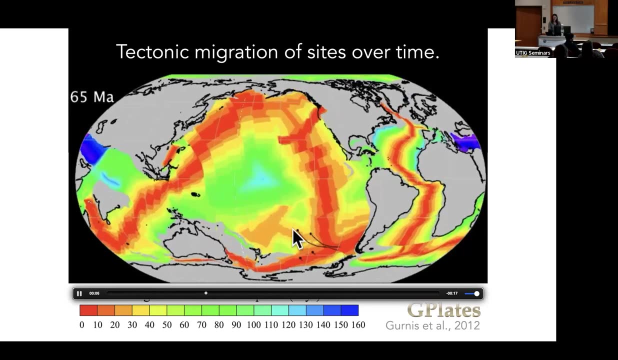 really comes from huge spreading ridges- yeah, cool. yeah, there's also- this is, uh in the modern day, like called the osborne trough, but it was an active spreading ridge- uh also that these sites kind of were in between these two bridges, so this hydrothermal material could have been coming from there or there, but then this range went extinct, um. 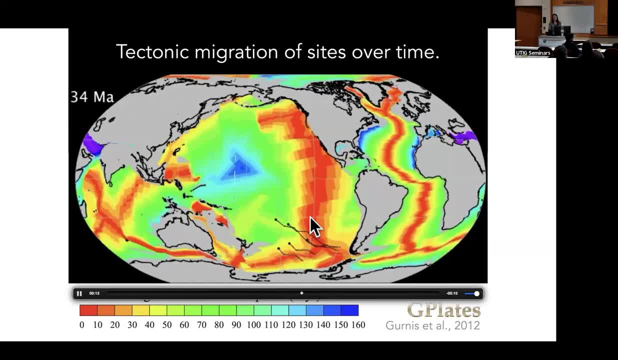 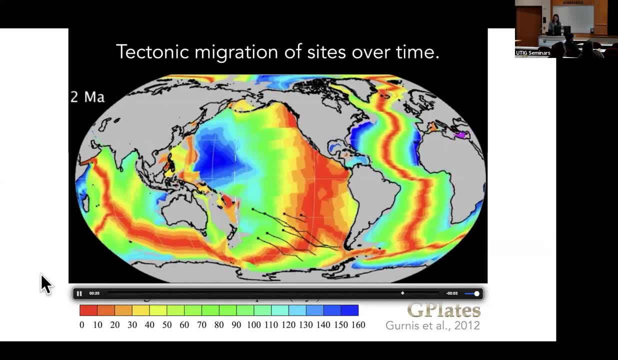 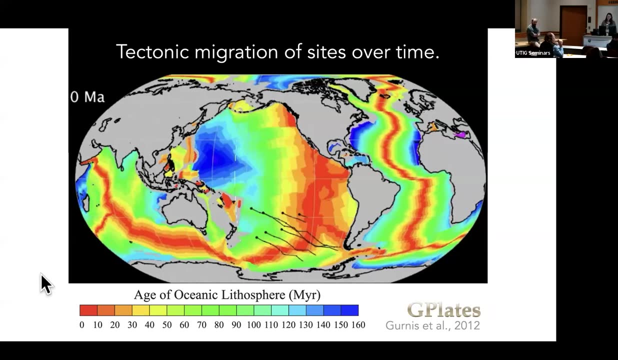 right around when we see like a drop-off in hydrothermal material. so that's my hypothesis as to why there's a bunch of hydrothermal material there. cool, that was great talk. um, i'm curious, just because it seems like it's going to really matter for this story that 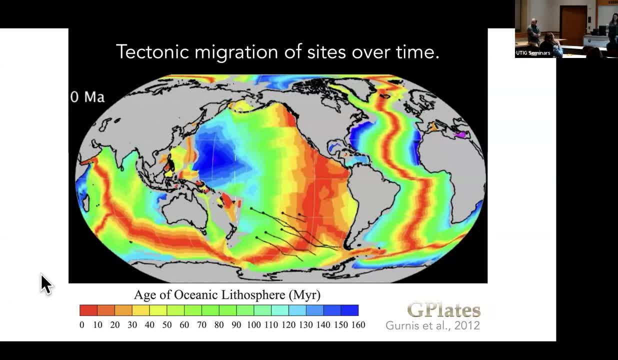 have we? has there been some thought about the distribution of really large scale rivers, and thus the delta generation, for the purpose of this reverse weathering component? i don't, um, i haven't seen those studies. uh, it doesn't mean they don't exist, um, but that would be interesting and just, and if there's a magnitude in that, then that that seems. 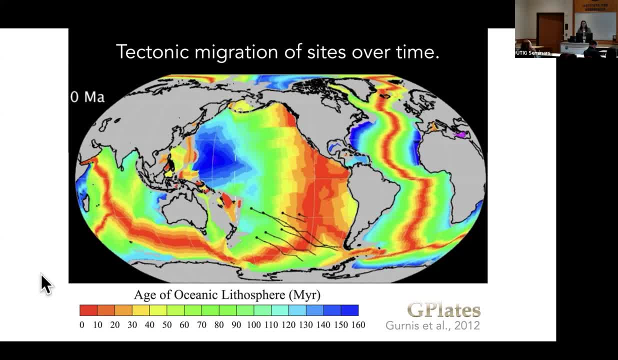 yeah, there's reasons for that. i don't know if there's a reason for that. i don't know if there's a reason for that, um, but um, it would be interesting to see. is there any evidence to indicate, uh, maybe it might have, uh, a large-scale, sudden transition from the? 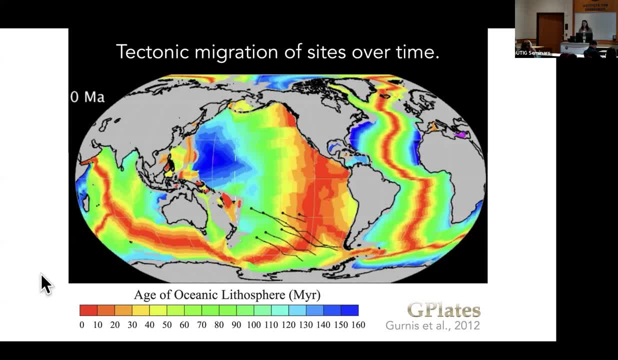 i don't know if that's the right word- what you're talking about in terms of like, what, uh, what's the method that you would be talking about? yeah, so i mean, i'd be interested to see if any of the other figures are based on uh, you know, like any of the other uh. 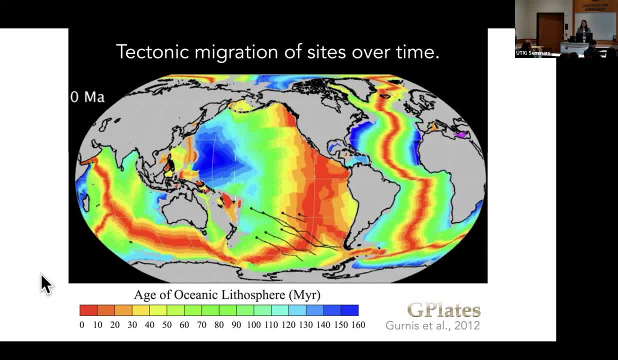 um, um, um, um, so, um, um, um, um, um, um, um. orthogenic clays, is one preferred over the other for generating a sink, um. so if you look at like images, like zoomed up of the diatoms or radiolarians, the clays like can. 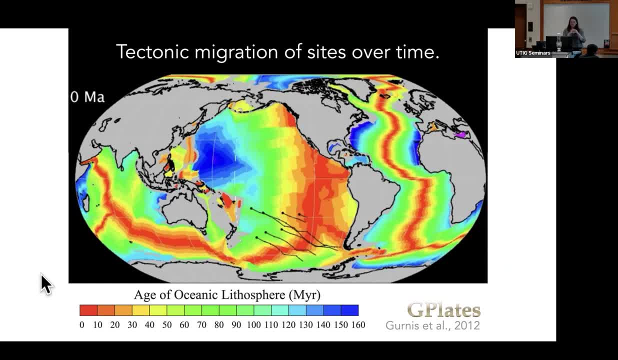 often form in like the pore space where you can really concentrate silica. so if there's like more or like- yeah, what do you call it? like divots, like the, they're almost enclosed, uh, in the the silica, um, i i'm not sure if one's like more conducive than there, that would be the. 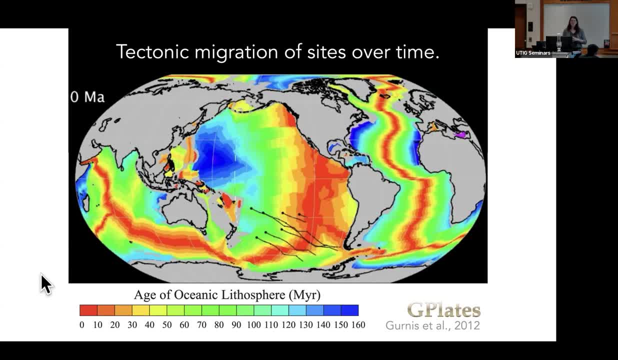 only thing i think of like physiological differences, um, for uh, yeah, i, i typically think about it more like a solubility difference. so if there's, if there's a solubility difference between them there might be, uh, the better preservation or the longer they can stay on the seafloor, the more likely i guess there is to make. 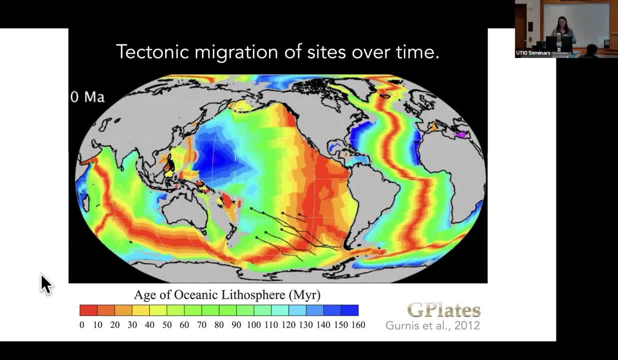 a clay? oh, because most of like silicon, the seafloor gets dissolved away um. i know these clays forming around these diatoms or radiolarians can reduce the solubility of them, so you also change the solubility as you make clay minerals around them um, which helps them stay on the 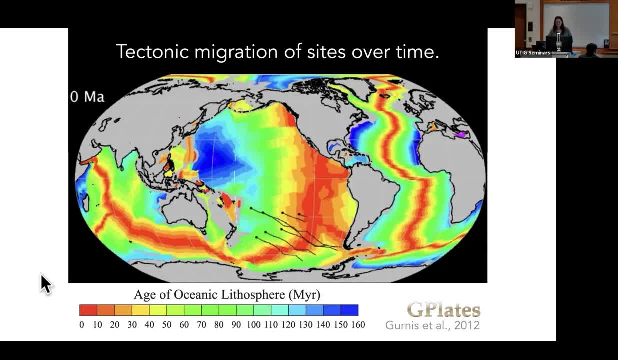 seafloor, uh, but specifically between radiolarians and diatoms physiologically? um, not sure. yeah, that's those are my thoughts on the topic. any other questions? okay, i have one too. um, so, thinking about like modern climate change and, um, you know, often silicate weathering is the thing that gets talked about as like on geologic time scales, the thing. 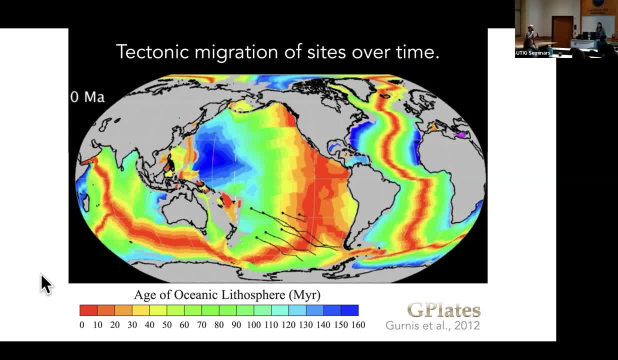 that'll bring us back to pre-industrial co2 values, um, and if, uh, reverse weathering is operating in opposition to that and it's not going to be able to do that, then it's going to be able to do it. i was just trying to work it out my head just now. when you're talking about that earlier, it's, it's. 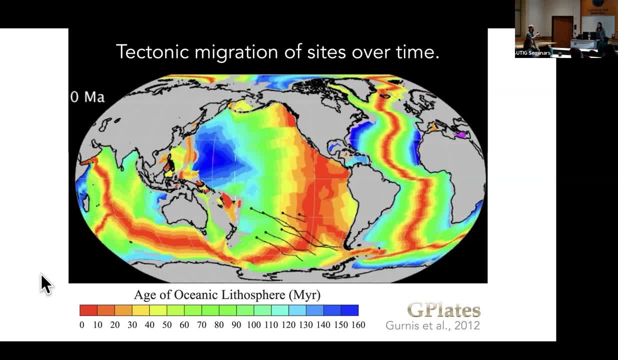 there's more reverse weathering when it's warming, right, i'm not sure there's been enough studies to say that it actually happens. but uh, uh, the controls on reverse weathering, i don't think they're well interested. i was saying for weathering, oh right, okay, yeah, yeah, so i was so. 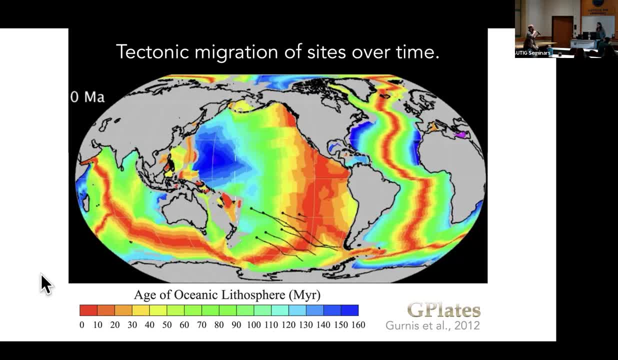 i guess. but my question is on a broader scale, like: so what? what will the role of reverse weathering be in that long-term drawdown of atmospheric co2 after the anthropogenic change in climate change? is it going to make it longer or is it going to be like extra cooling? 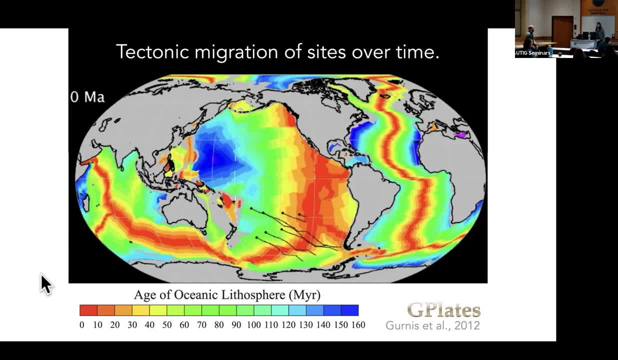 that happens afterwards, or what do you think that's a great question. um, i'm not sure. i mean the reverse weathering and it's like implications on like climate are not well understood like right now. so right, oh, that's what's exciting about like a new thing, like a 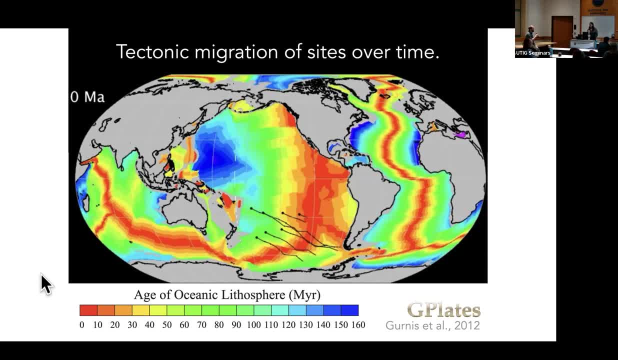 new, a new part of your system to quantify, right? so, yeah, cool, um, okay, well, if there are no further questions, um, we will be going, uh, to happy hour at Austin. Beer Works around four and everyone is welcome to join us there. they, of course, have a roof and walls.